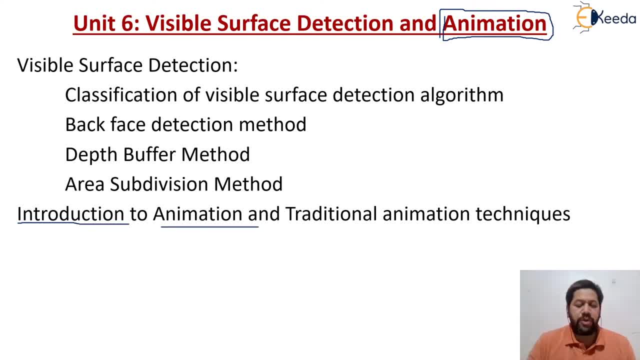 introduction to animation. We are learning basics of animation, or introduction to animation, and we are also going to learn the traditional animation techniques, Okay, which are the steps which are used in the animation and we call it as our traditional animation technique. Okay, so today's, our topic of discussion is introduction to animation and traditional 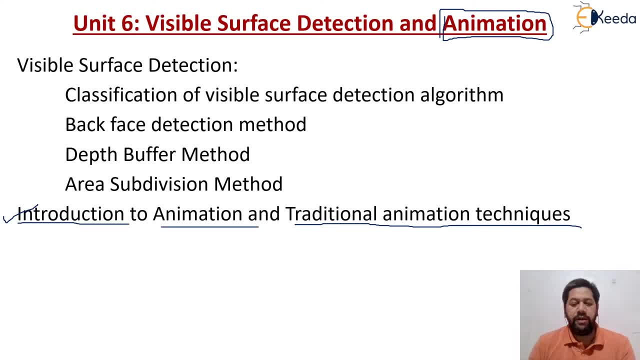 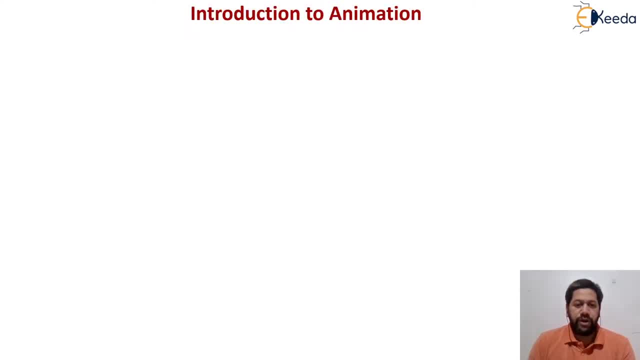 animation techniques. Okay, I just moving to the next slide. Okay, so that we can start our discussion Of the introduction to animation. Okay, so let us start understanding what is mean by animation and what exactly are where it is applicable. Okay, so we are considering the general applications. 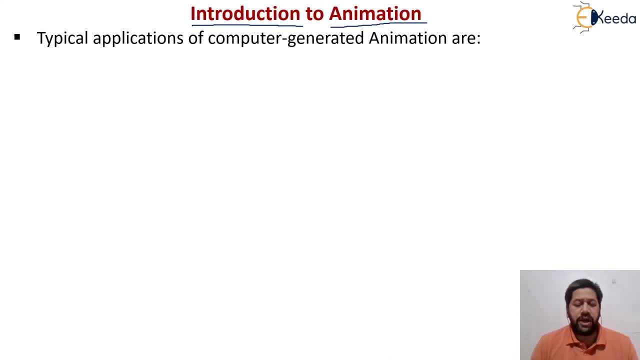 of the computer generated animations are okay, but we are understanding where exactly the animation is useful and which are the application of animation and that's why, why this point is important and we are learning this point under the computer graphics Okay, which are this general application that we are having of the computer animation. See. 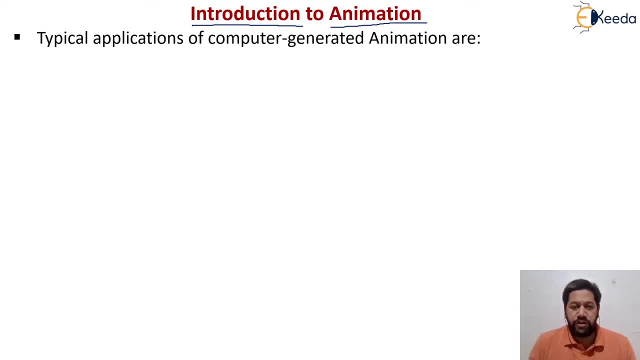 and Instead of using the word here only as an animation- Okay, you stop using only one as animation. We usually use the word as computer generated animation. Okay, because all these animations are possible with the help of the computer and computer graphics. So we are calling. 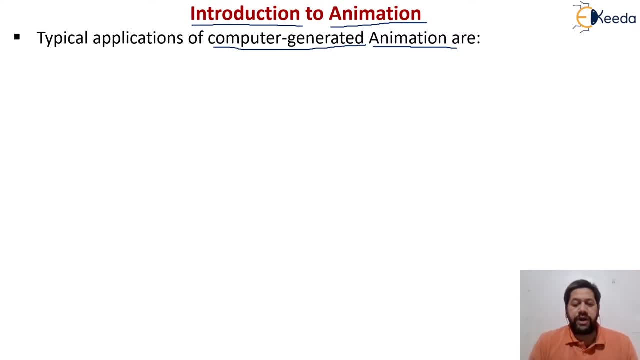 it as it is computer generated animation. Some of the textbook refer it as a computer animation. Okay, so that's why I'm using this word as computer generated animation. Okay, so that's why I'm using this word as not only animation. 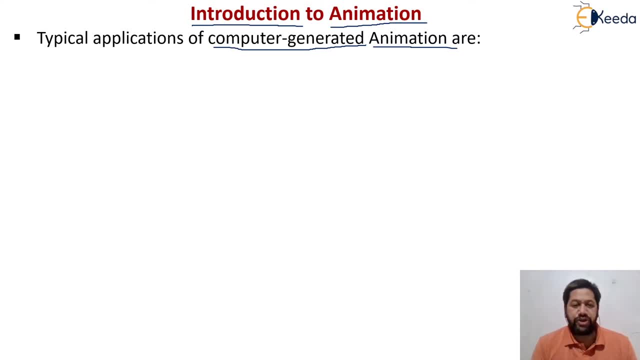 I'm using this word as a computer generated animation. Okay, which are these? application to the first application, as it is known to everyone, is that is, we call it as the entertainment. Okay, in entertainment industry or film industry, We are doing that. there is the huge scope. 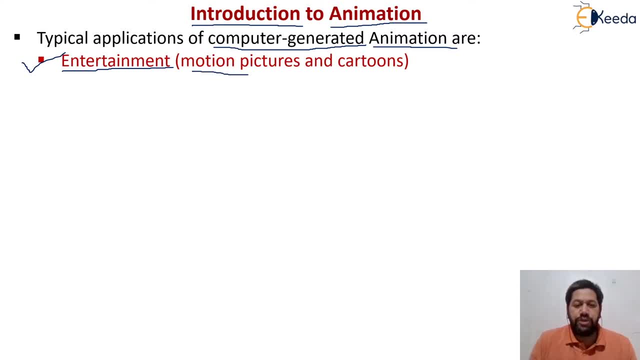 for the use of the animation: Okay, so it will be using all these motion pictures. Okay, what will be are knowing about all different types of picture, as well as a as in maximum time. It is also used in the cartoons. Okay, so in animation is very useful in all the types. 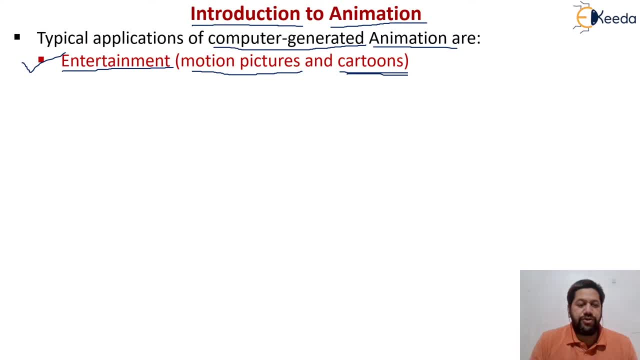 of the cartoons. Okay, so that we are considering the first application of the animation is entertainment. No Second application that we are considering it is in the advertising. Okay, we can find that nowadays there are so many advertise Okay which are generated with the help of the animation. 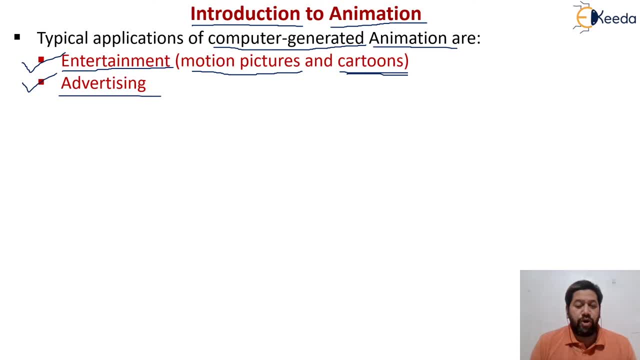 Okay. so we are having some different object, Okay, which are not maybe the real-world object, Okay, but the objects are animated and we are showing so many things in the advertisement with the help of the animation, Okay. So the second important application. 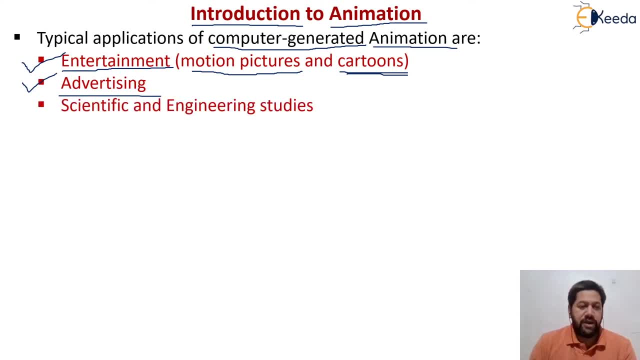 or the area where animation use is the advertising. the third one, as all of you are knowing, to the scientific and engineering studies. Okay, See, whenever we are going to learn so many different working of any particular, we can call it as maybe suppose I considered in atom oil industry here. 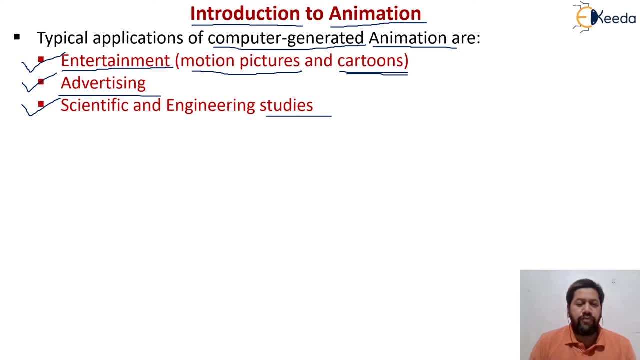 or mechanical engineering, electronics engineering, So all the working of different technical concept, Okay, we can study, we can visualize with the help of the animation as well, as it is definitely used in the scientific studies also, Okay, related to medical science field here, so that it will be more easy if we generate the animation. 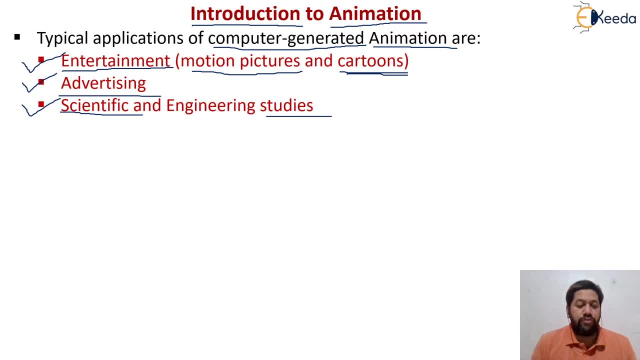 Okay, or whatever the concept that we are going to put in front of everyone, that will be with the help of the animation. Okay, So this is the next application and obviously, as we have learned in the computer application, I think the fourth very important thing that I consider it is it: 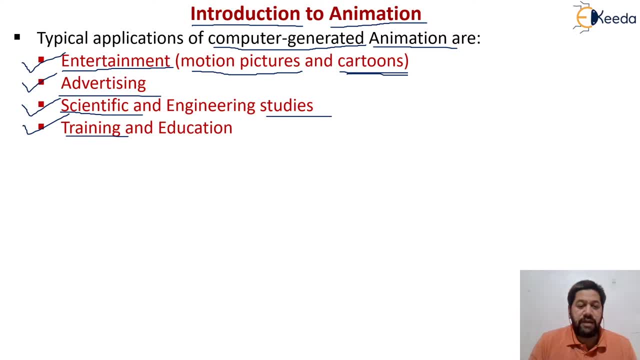 with. nowadays, it is useful in the training as well as the education. Okay, it is using training and education. Then you can find: nowadays, There are so many online applications or online classes are there for the kids. Okay, so maybe for the students. 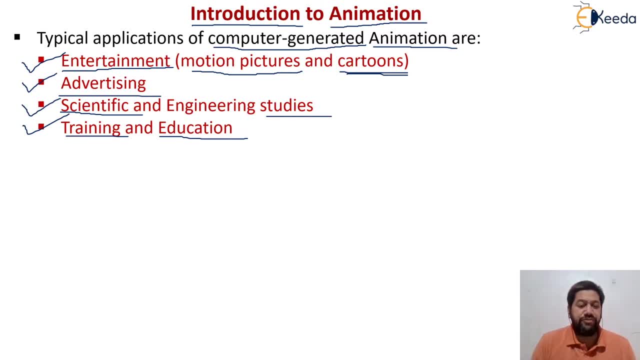 which are maybe just studying into the lkg-ukg for standard. Okay, all now you can find that they are Learning this with the help of the different cartoons also Okay, so they are learning ABCD. They are learning all these with the help of this animation. 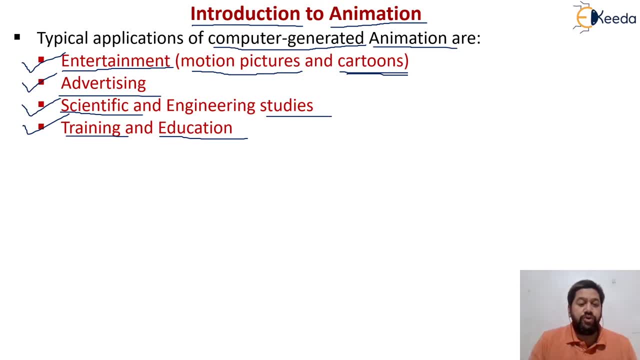 I see the main important nowadays. It is also useful in all the type of the training as well as it is using the education field. Okay, So these are the different applications, or these are the different areas where the animation is useful and the animation is applicable. 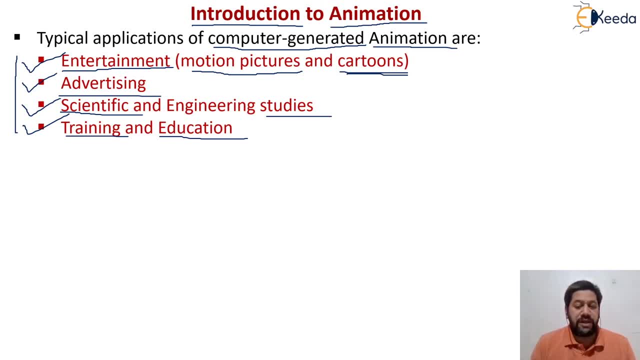 So that's why our today's topic of discussion: We are learning what it means by the animation and what is my Basic technique behind the animation that we are using. Okay, so it is continue our discussion. I hope all of you understood. 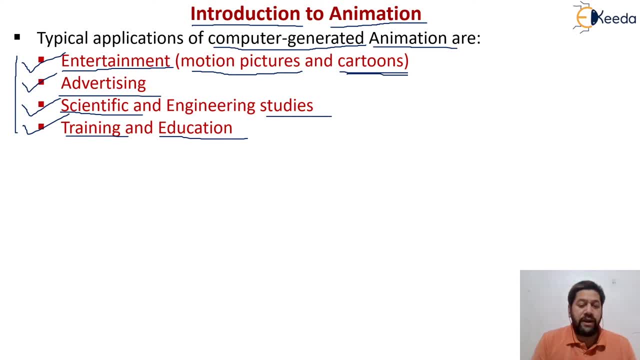 These are the areas where animation is used. to understand what is how I can define animation now. Okay, So I see that the computer animation generally refer to any time sequence of a visual changes in the scene. Okay, so computer animation refers to any time sequence. 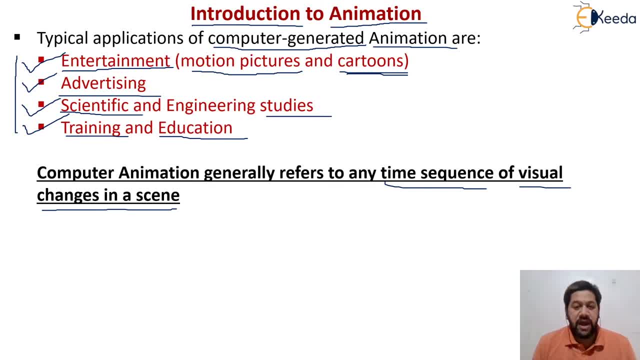 So we can find that there are so many sequence, Timing is there and, appropriately, we are generating the frames, The frames are displayed, appropriate timing, Okay, and it is going to create some motion. It is going to create the visual changes into the scene. 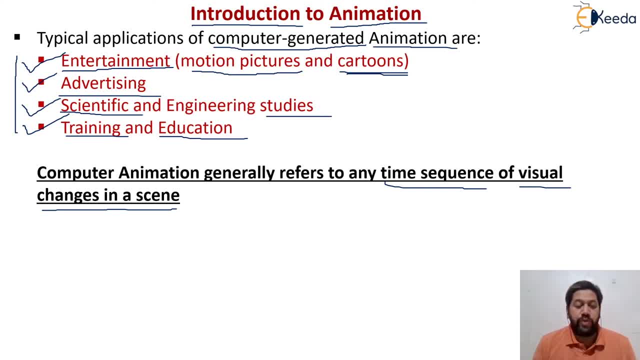 and it is more easy for understand or for us to visualize it. Okay, So that is what we are considering as it is animated, All the things that we are considering as the animated. Okay, So this is what we can say- refer to the basic definition. 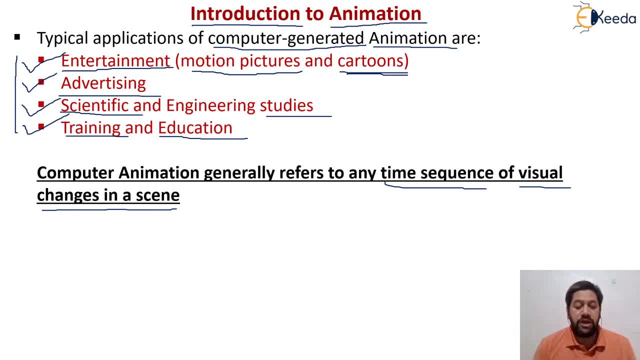 So computer animation generally refers to any time sequence. Okay, we are applying the time sequence of a visual Changes in the scene. Okay, so if the scene we are applying this time sequence and we are finding that visual changes in the scene, Okay, I think you have seen all the old movies. 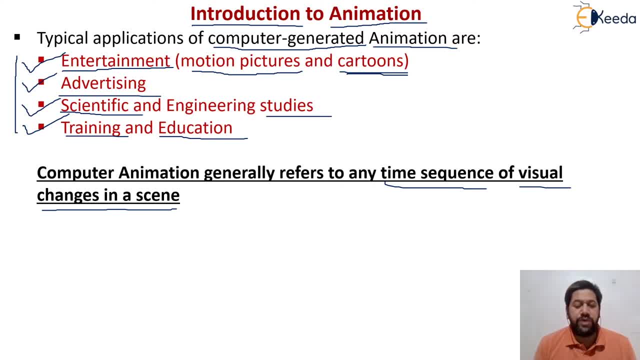 Okay, I'm not talking about the recent movies. If you can see that, the old movies, you can find that okay. the hero or the heroine, you can find their driving the car- Okay, at that time that animation industry has not. that was developed. 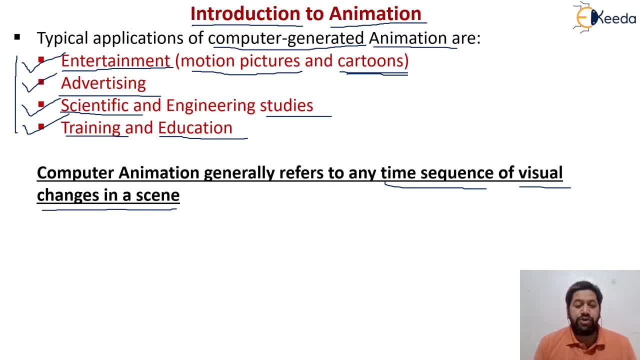 Okay, they have not that much research on it, So you can find that what is shown over there is maybe the car and the hero and the heroine, those who are driving it. Okay, we are sitting inside the car. I think that car is not going to change, only the their background. 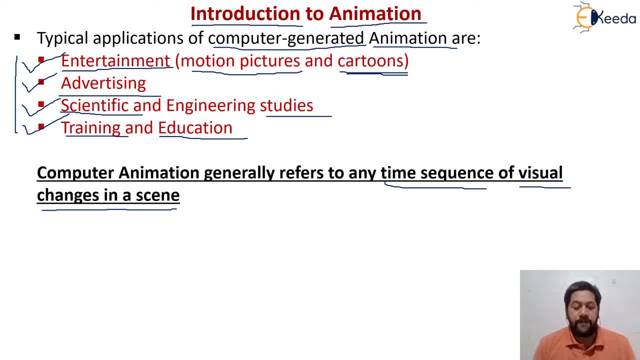 scene is going to change and we will feel that they are driving the car Okay. So all such things are there, but that was initial stage. But nowadays we are having so many research and too many additional things are there in the animation which had made this animation industry. 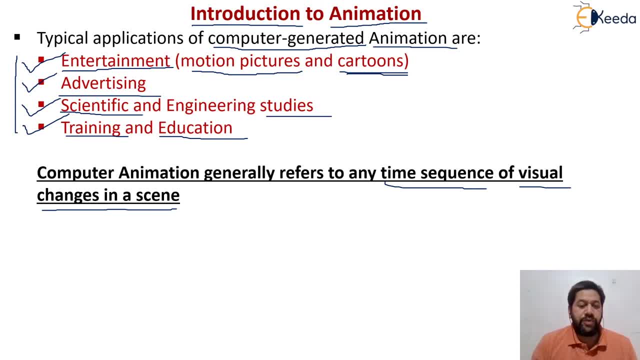 as a complete, separate area of research. Okay, So that is what we are talking about: computer animation Now, in addition to changing the object position. So that was I told the first. generally, what we go for is we are going to change the object position with the help. 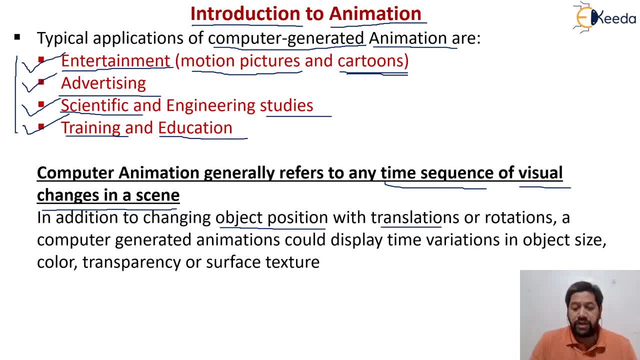 of, I think initially we have learned we can change the object position with the help of the translation or rotation, a computer generated animation to display time variation in the object size. Okay, So now we cannot apply only translation, rotation, but we have to display the time variations in the object size. 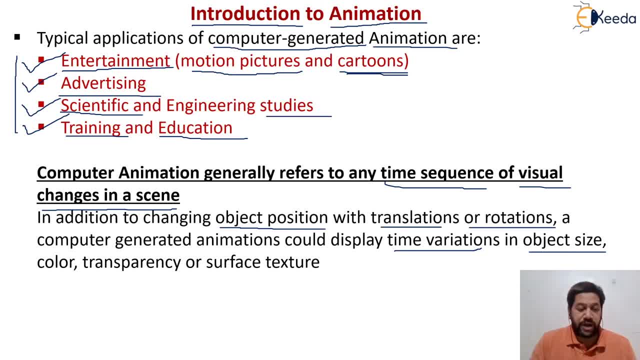 Okay, we have to display it with the help of the, not only in the size of the object. We have to show the time variation, the color, in the transparency or the surface of the texture of the object, everything We can say that it is going to change with respect to the time. 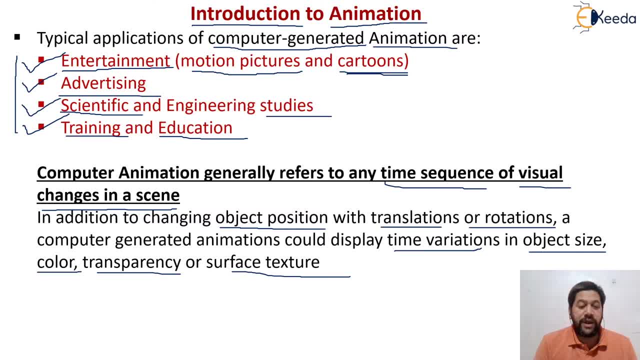 Okay. and the time variations- We are all time sequence- are added here to make it as a animation Okay. No, you can find that advertising animation often perform the transition of one object shape into another a maximum time. We can find that in the advertising. 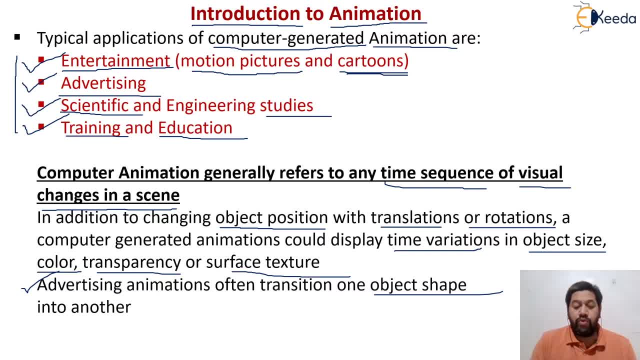 animations, we can find that there is a transition, is always there and we are going to check the shape of the object from one object into the another object. Okay, So initially I'm having this object. If I use this, it will directly change into this. 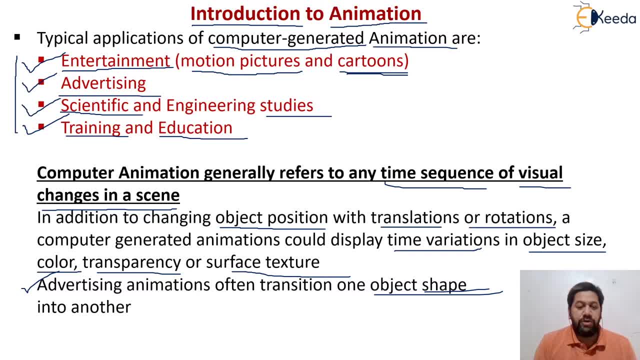 Okay, so that all such advertisement area, looking, you can find the area where the transition is there from object shape, from one object to the another object, and it is that transition is very smooth and we come to that, Yes, object is directly converted from one shape. 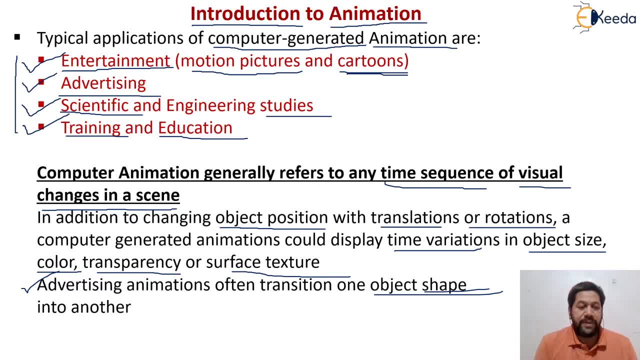 to another shape and so on. Okay, So this is what our basic things related to the animation, For example, I think there are so many advertisements are there. We are can consider the example, but just I am considering that transformation of a can of motor oil. 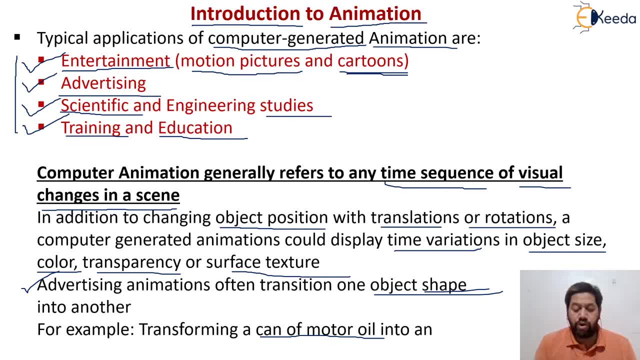 Okay, so I'm having just one engine oil, or the motor oil I'm having, and you can find that with the use of this, or they can show that it will be converted directly into the engine. Okay, so many things are there in the advertisement. 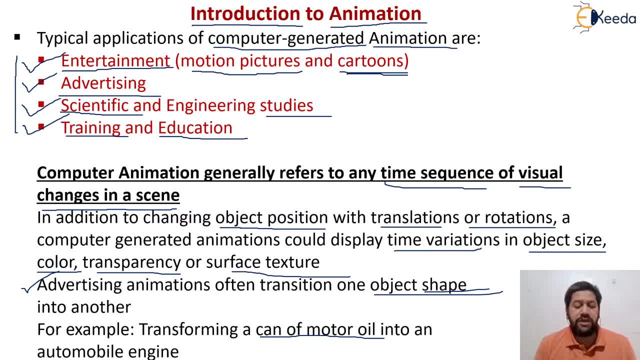 We can watch it as how it will be useful. Okay, minimal it possible. We can see the one more diagram also to show that how this animation is displayed or it is works Okay. So I consider this is a very basic thing related to introduction to animation under this part. 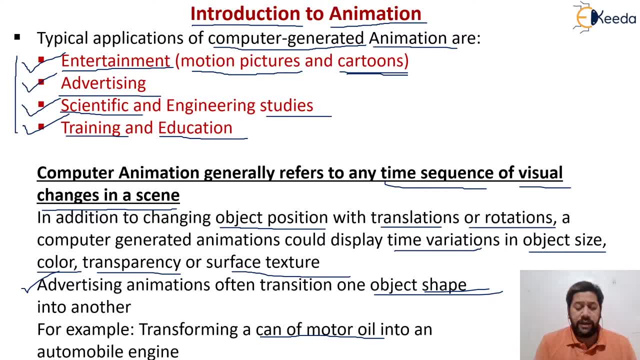 Okay, Now we are considering which are the other varieties of animation which are possible. Okay, so I'm just showing you which are the things which are possible in the animation, or how I can perform the, or how with the computer graphics, how I can achieve with the animation effect. 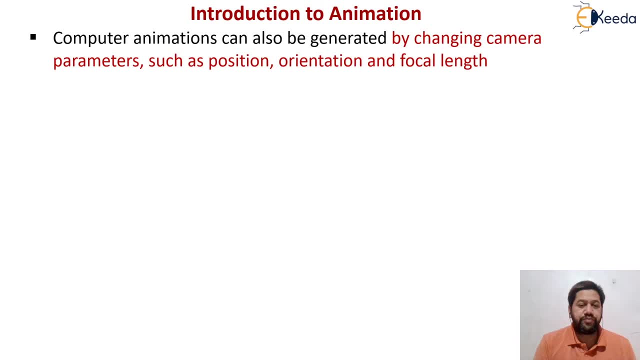 Okay, so just moving to the next right now. Okay, so here you can find the computer animations can also be generated. computer animation can also be generated by changing the camera parameters. Okay, so you can find that in so many nowadays videos are there. 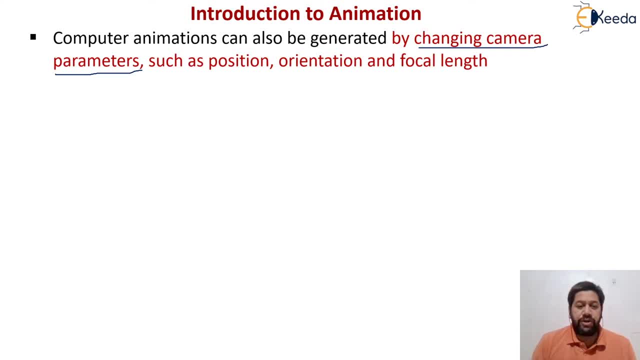 Okay, you can find that the they are changing the camera parameter, They are changing the position of the parameter. They are changing the orientation of the parameter. Okay, as well as they are changing the focal length. Okay, you can find it. so many videos. 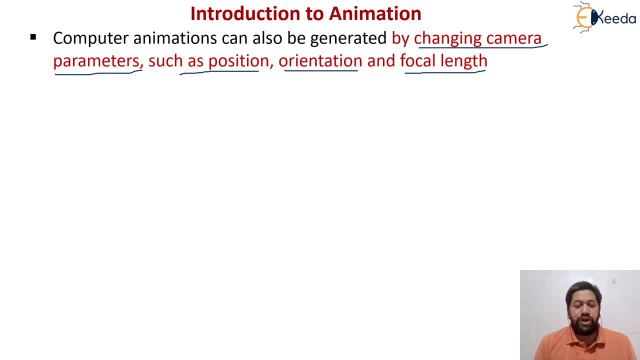 You can find the position is changed. It is not straight. It may be with the different angle. It is shown. its orientation is shown. its focal length change. Sometimes they focus, will go to the more closer to the object or that particular person. Sometimes will be at the different time. 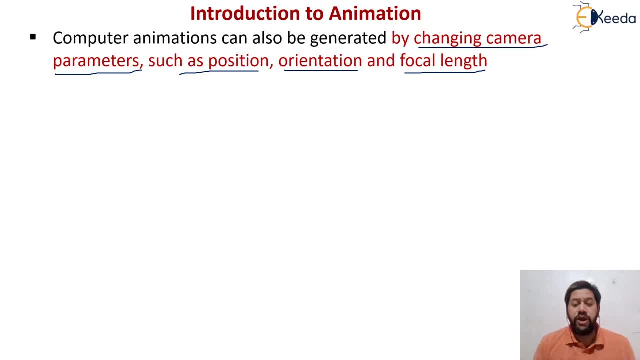 and they are very good, Okay. So all these things you have seen nowadays into so many videos, Okay. So first thing I'm just mentioning here: in the computer, animation can also be generated by changing the camera parameters Maybe, such as the position of the camera orientation. 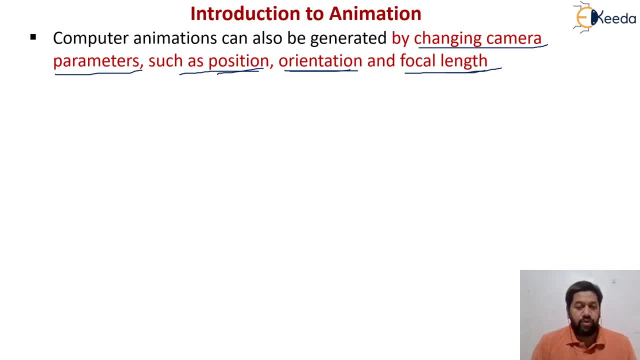 of the camera, focal length of the camera, Okay, and so on, so I can in a position to generate those animations are possible, Okay, second, we can produce computer animation by changing- Okay, I had told animation is produced here in this cases, or point number one can be produced. 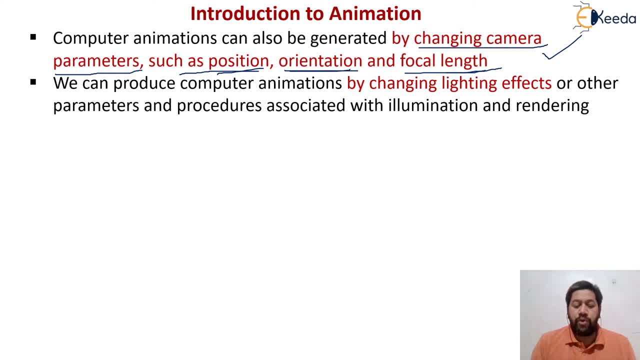 with the, by changing the camera parameter in second, What I'm showing, produce the computer animation. now, by changing the lighting effects. Okay, by changing the lighting effect or other parameters and procedure which are associated with the illumination and the rendering, I can also produce the animation. 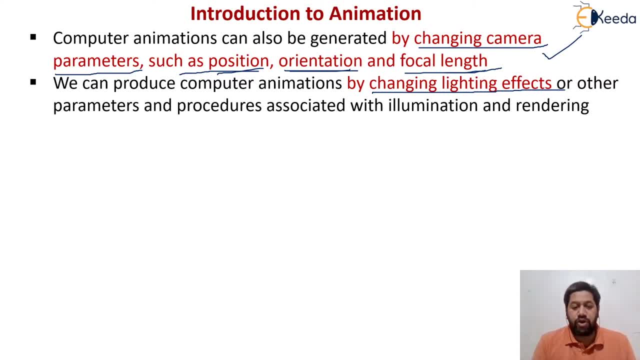 Okay, So just by changing the lighting effect of that particular picture. Also, it is possible for us to create the animation. Okay, that is what I have mentioned, or we have mentioned here. No, there are the many application of now here. 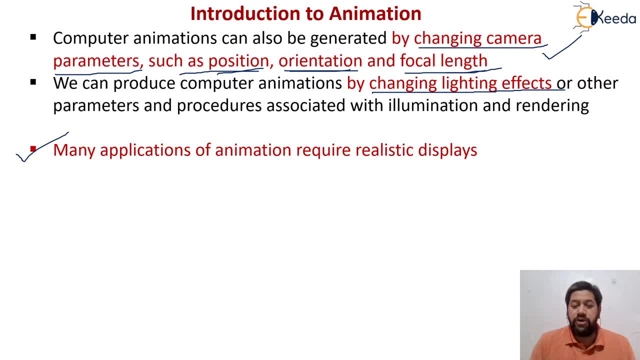 I think this is very important. many application of the animation required a realistic display. Okay, So many things are there where they want to use the realistic displays, not the computer-generated objects will always use if I'm talking about cartoon, Okay. So whatever the different series, 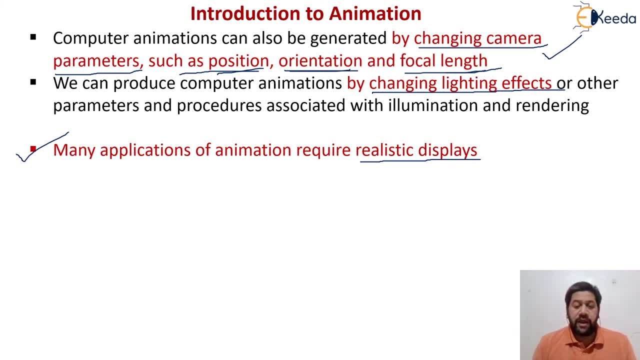 or we can see the pictures of related to the cartoon We are finding. Okay, actually it is the computer-generated object. Okay, maybe the Mickey and Mouse? Okay, whatever we are considering, do many different cartoons are there? this cartoons are generated, all these objects. 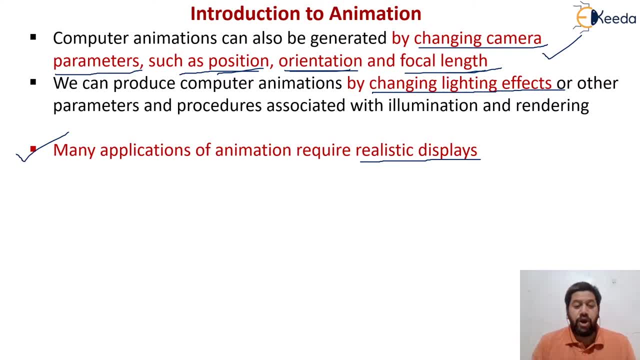 in that cartoon are generated with the help of the computer. Okay, but here I say I just want to mention that there are many applications where animation required. the realistic displays are required, not the computer-generated objects We are using in the animation. Okay, so that is what the point I mentioned. 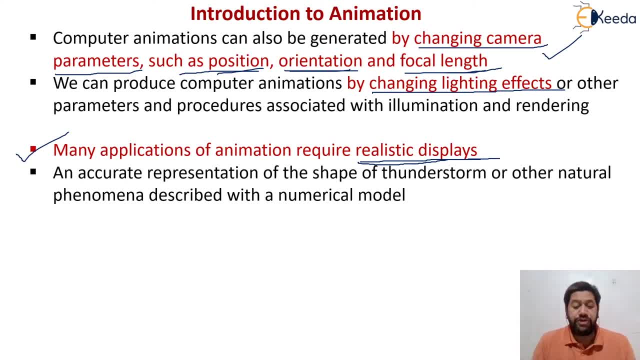 and if I'm having the realistic display, if I'm having the realistic view in my animation- okay- then the accurate representation of the shape of the thunderstorm or other national phenomena described with the numerical model will not be work. Okay, so we have to show this. it should. 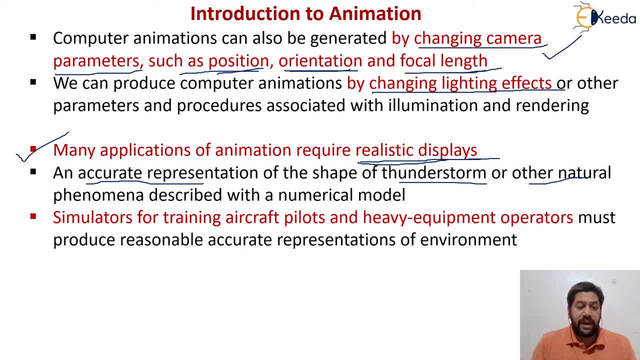 Look at the realistic. Okay Now. for example, I just consider that I think we have seen this example in the while learning the application of the computer graphics, We know that there are the different simulator which are for training the aircraft pilot. Okay, so whenever the aircraft pilot is going to get the training, 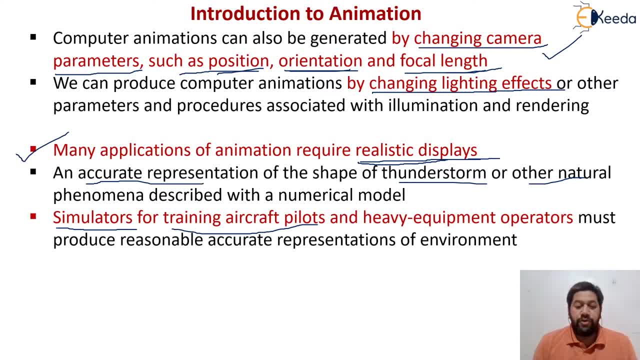 I think cannot drive directly the aircraft or the plane directly, So it will get the training with the help of the simulation. Okay, and we have seen that that simulation not only applicable for aircraft pilot, but that simulation Is applicable for heavy equipment operators. 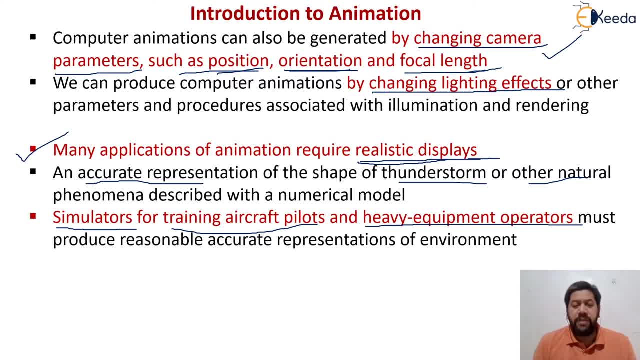 Okay, so those who are having- I call it as not only the JCB- may be very small, Okay, but so many heavy equipments are available and all these operators should be trained not only directly on that equipment, but they should be trained on the simulation. 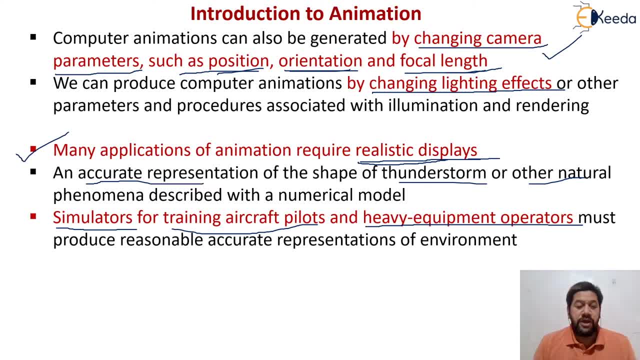 Okay, I think I have explained in some of the previous lectures that such animation or training for the pilot, training for the heavy equipment- I think they are sitting in the room and the room is completely surrounded by the different screen- Okay, and they are having in front of there. 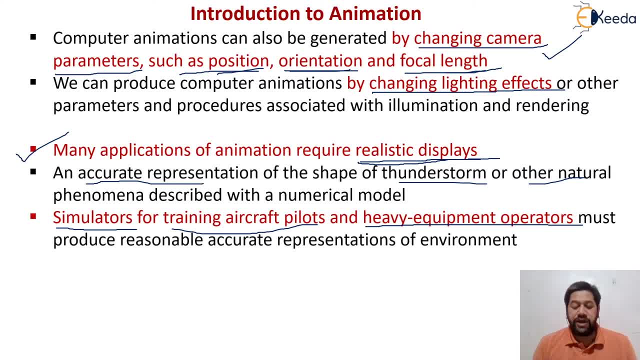 They are having the panel- Okay, control panel is there as they are changing, as they are moving. Okay, maybe they are shifting to the gear. They are changing the direction of the airplane or the aircraft automatically. what we need to show that the scene- okay, behind there- should be changed. 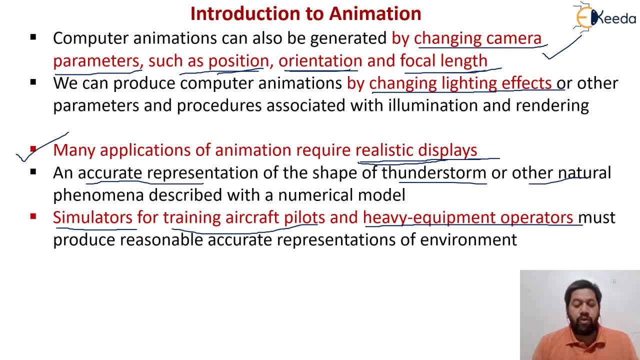 Okay, front view side views. everything should be changed and all these things are animated, Okay, and if I am having the animation which is related to such simulation, Okay. what I want is I want my object shape should be represented appropriately. So that's why we are written most: produce the reasonable, accurate. 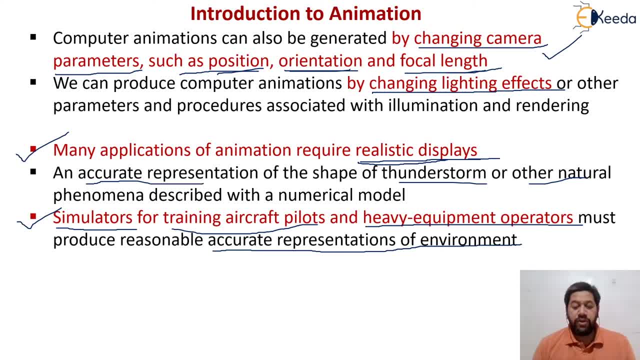 representation of the environment. Okay was, as the surrounding environment going to change from the environment changes and accordingly, we are considering it as it is using the animation. Okay, so I've explained so many different types of animation which are possible for us. Okay, so let us continue our discussion. 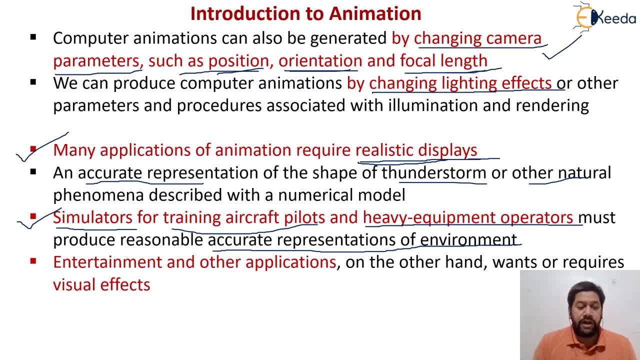 Now, if I talk about simulators, okay, but if I am talking about the entertainment application, okay, so I'm just going to this point. entertainment and other application, on the other hand, wants or requires a visual effect if they don't want the accurate representation of the environment. 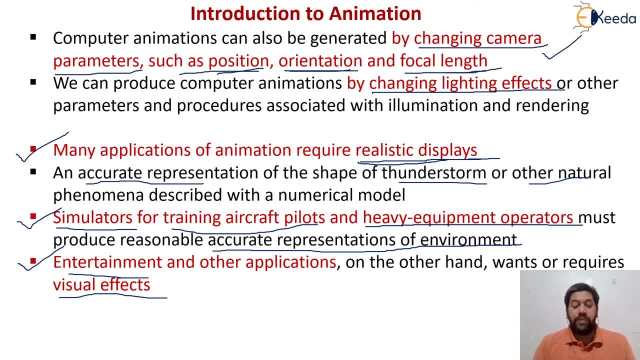 but they want, okay, maybe entertainment and other application they may want. the animation should provide them the correct visual effect, Okay, or they are more interested into the visual effects and so on, Okay. So this is what we are having, considering that, which are the different ways. 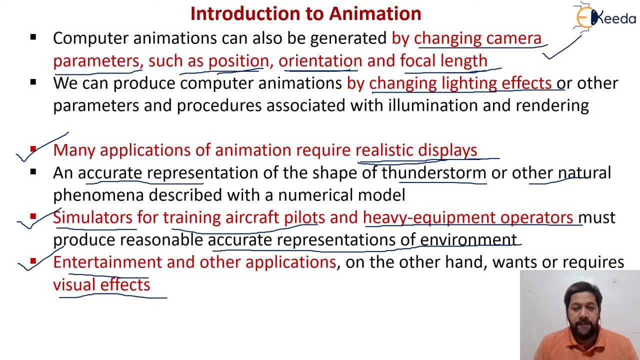 Okay, or the requirement is there related to the animation that is shown over here? Okay, let us continue our discussion Now. therefore, in animation: Okay, scenes may be displayed with exact rated chefs and unrealistic motions and the transformation: Okay, so all the things that we have to use in the animation. 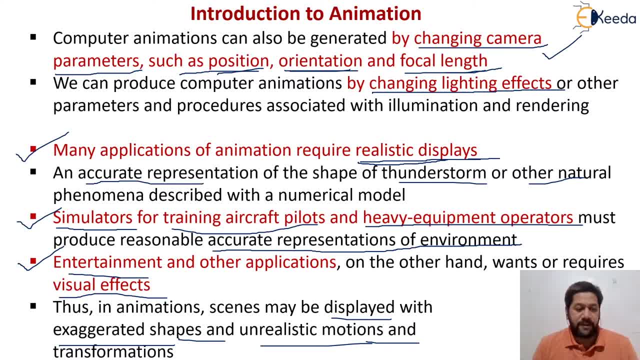 and that is what this point going to consider, or this point explains, Okay, in this particular case. Okay, so let us move now to understand- I think we have learned- What is the basic of animation application, how I can provide the animation. Okay, maybe by changing the camera. 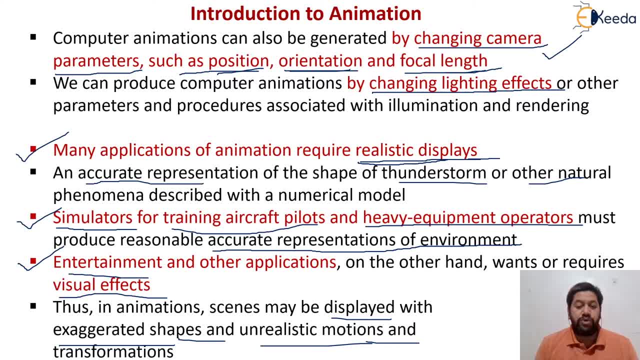 maybe changing the lighting effect. Okay for realistic image. Also, I want the visual effects will be changed for simulators and all such animation. I want the accurate representation of the environment of the object should be there for cartoon and all. we want that computer generated object should be moved. 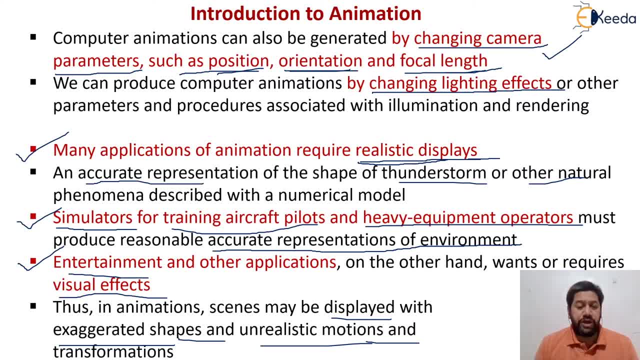 They automatically, and so on. Okay, let us continue our discussion by understanding the next point, I think where we are going at the end of the session. I'm going to show you the different animated images. Okay, but initially let us focus on learning. 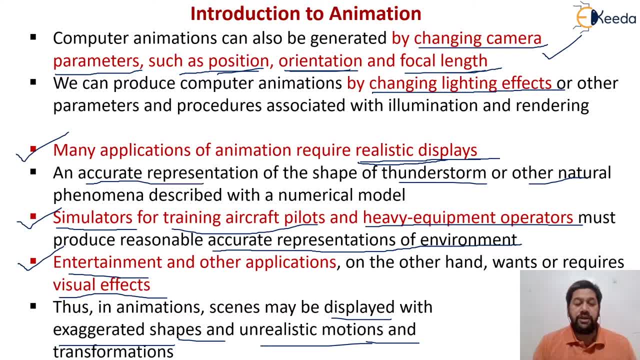 which are the animation techniques? are there? Okay, I may call it, as these are the traditional animation technique, but we should understand which are these animation techniques are there? Okay? so let us move and continue our discussion. I'm just moving to the next slide now for the further discussion. 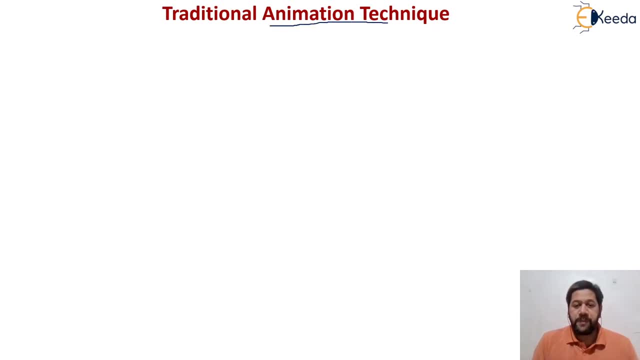 Okay, so let us understand the animation techniques. Okay, Now our focus is on Understanding the animation technique and know why I'm using this word as a traditional. because, as I told, nowadays, okay, there is so much scope, so much improvement, Okay, so many variations, so many research are there. 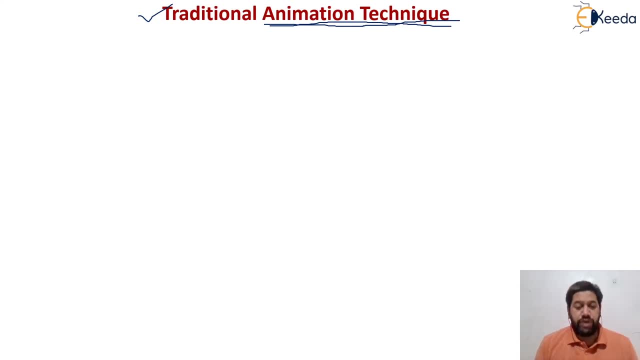 in the animation nowadays. So, whatever, just now everyone is using I call it as the a recent animation technique, but now we are just focusing now on traditional animation techniques to understand the basic, Okay, related to the animation technique. So that's why I'm using this word as traditional animation. 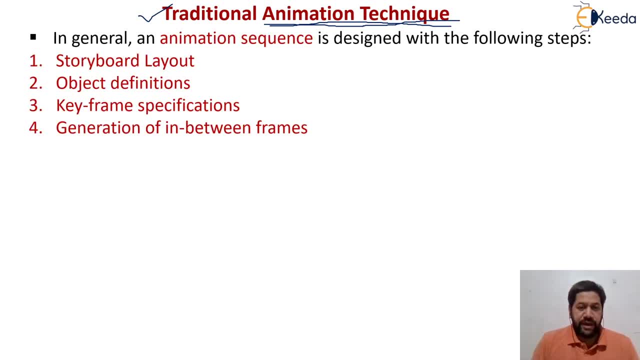 Okay, so let's look at the different techniques now in general. okay, and animation sequence is designed with the following steps: Okay, because we have learned in animation What we have to do. we have to generate the sequence- animation sequence or time sequence we have to generate. 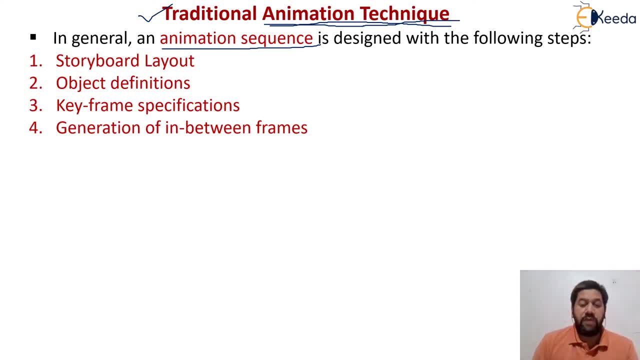 Okay, So now, to generate this animation sequence We have to follow, following these steps. Okay, which are this four step here to follow? the step number One is storyboard layout. Okay, what I have to design? I have to design the storyboard layout. second, after it is over. 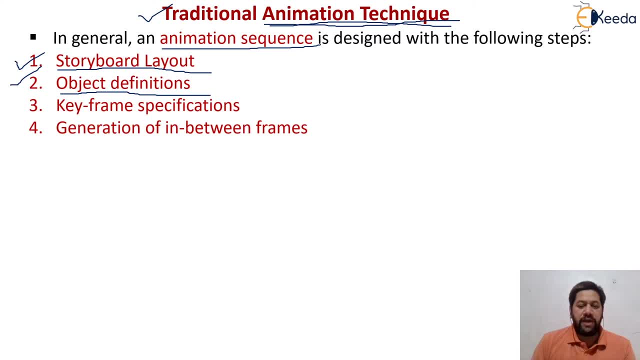 I have to define the object definitions. Okay, I have to define the definition of the object. the third and very important thing that we have to do is we have to go for keyframe specification. Okay, third step is keyframe specification. I think we are learning this: keyframe specification. 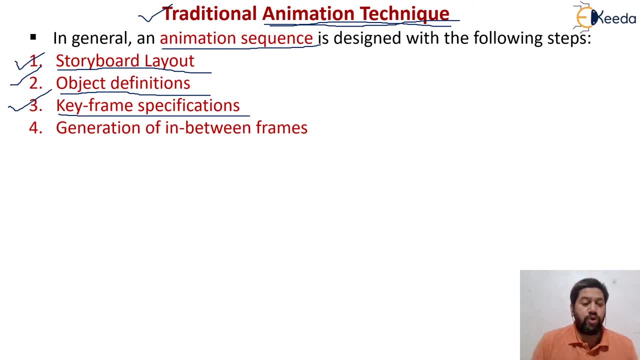 in a separate session, Okay, where we are going to have more focus on the keyframe specification and the fourth step that we are calling it as the actual general Generation of in-between friends, Okay, or actual generation of the frames I may require. some in-between frames are required. 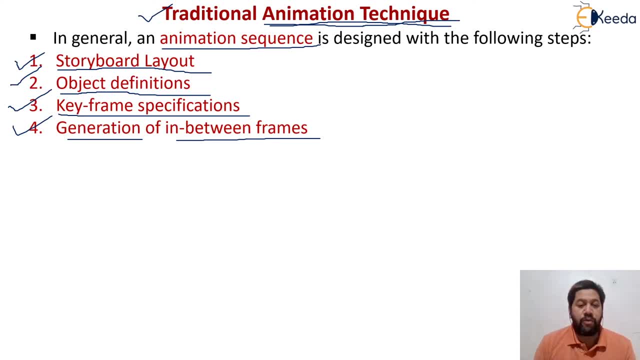 Okay, for the motion picture, or to show this as in the form of animation? Okay, So that's why I am considering now. These are the four steps that I am going to follow- Okay, in general, for the animation segment. Okay, So let us. I think we should understand this techniques one by one. 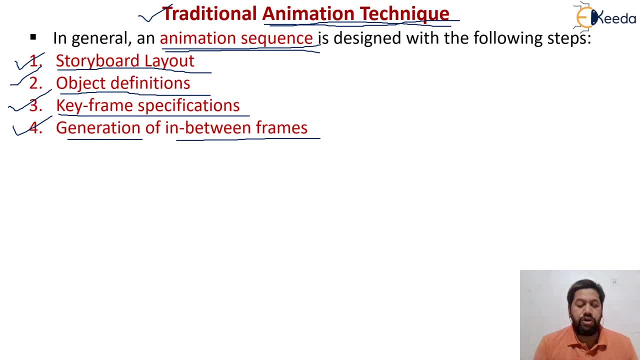 Okay, So, but before we are going to this, we just continue our discussion over here, And then we will understand these four steps one by one. Now this standard approach for animated cartoons. Actually, we can say the four steps are more applicable for generating the cartoon animated films. 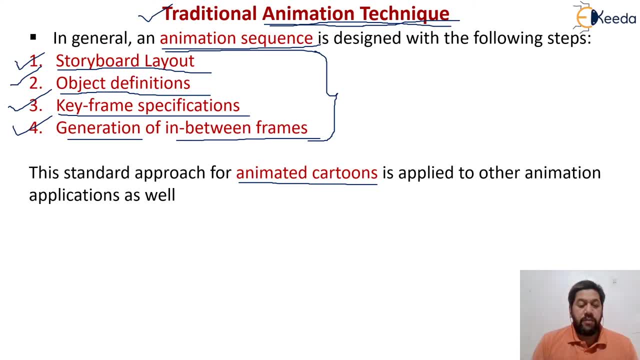 Okay, cartoon films Okay, or cartoon scenes, but the standard- this is the standard approach- actually is used for the animated cartoon, but is applied to other animation application as well, by say: these are the Four steps are applicable everywhere, But initially all the steps are designed by considering the animated cartoons. 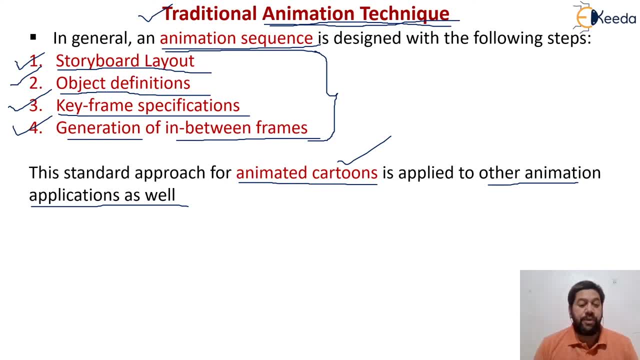 in front of them. Okay, but this is nowadays applicable everywhere. So that's why I'm calling it as a traditional and the basic method that we have to follow, and we have to consider these steps. Now for frame by frame animation. okay, frame by frame animation: each frame of the scene is separately generated. 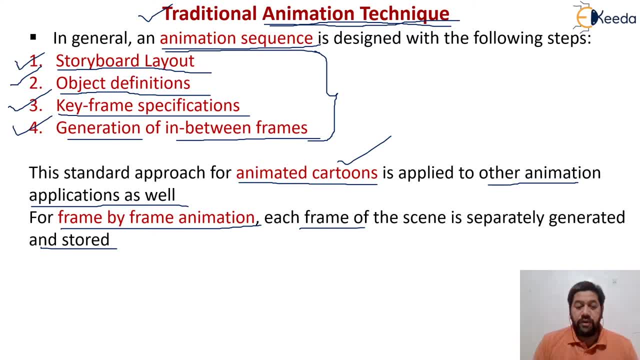 and stored. see, you can find that in I'm generating the animation frame by frame. Then each frame of my scene, every frame which is shown in the scene, is generated separately and it is also stored separately. So all these frames are stored and generated separately. 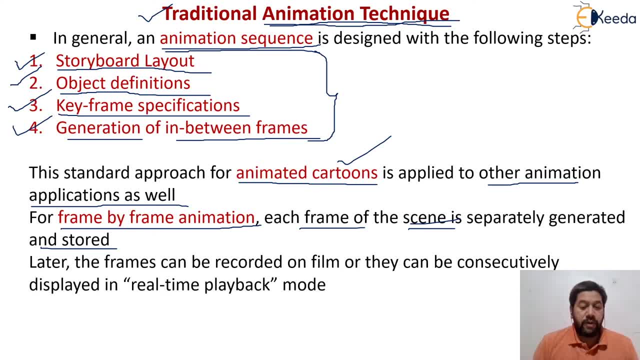 That is what I have to mention here later. Now, after generating the separate frames in my scene, okay, later the frames can be recorded on the film or they can be consecutively displayed in your real time Playback mode. after generating all this frame, 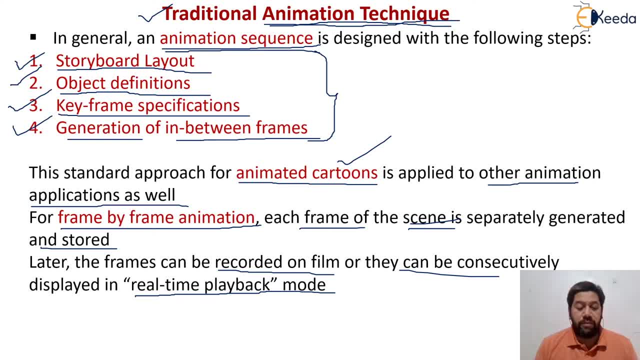 I just had to what we have to do. the frame can be recorded on the film, So we have to record it as in the form of the motion picture, We have to record it as a film and that can be consecutively displayed in a real-time playback mode. 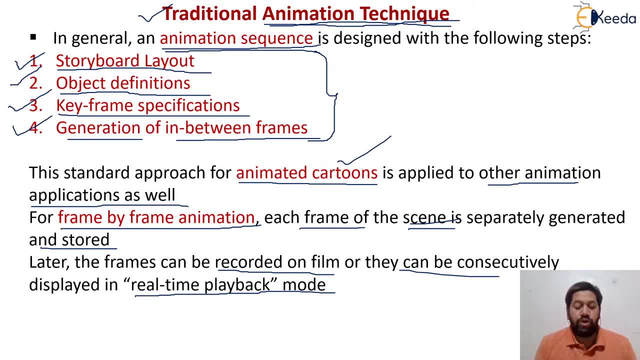 Okay, we are time, we have to play all these frames or display all this frame in a time sequence, and that is what is going to form my animation. Okay, so I'm having. so I just want to mention this point is: I'm having a number of frames with me. 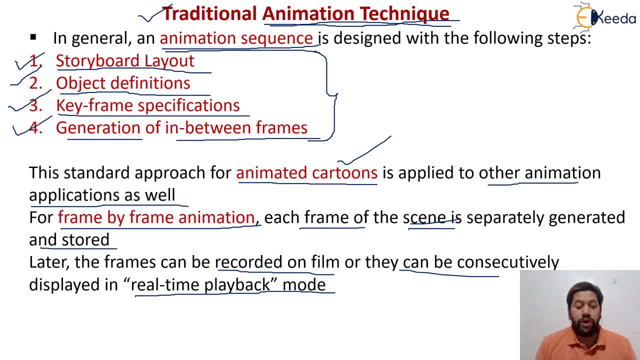 and all these frames and going to display. Okay, I'm going to record in a time sequence way and that is going to form me the motion picture, or that is going to call me as an animation. Okay, So this is what we have learning. 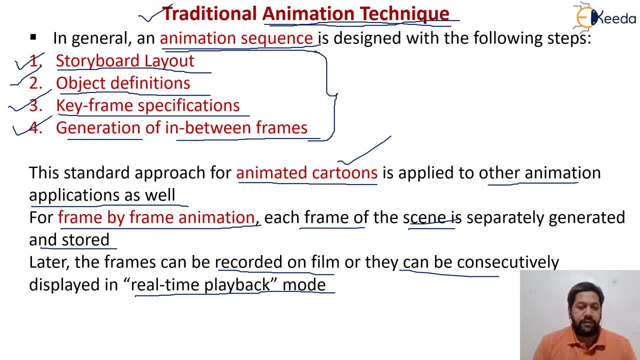 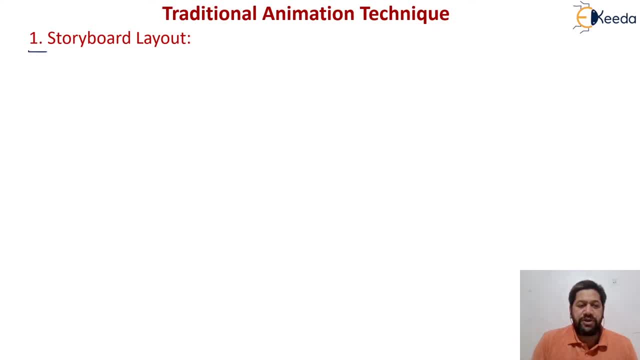 or we have mentioned in this particular slide. Okay, Now we are going to learn this four step, one by one. Okay, start learning this four step one by one. What is my step number one? Okay, I'm just highlighting my step number one. 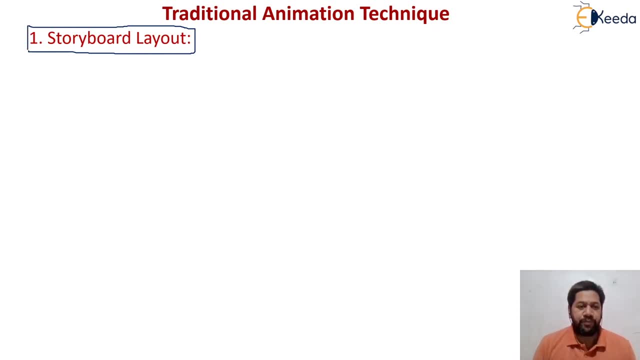 See, my step number One is story Board layout. okay, storyboard layout. I think the name itself indicate that I have to lay out my story on some scene or some board. Okay, so that will call it a storyboard layout. So that is my step number one. 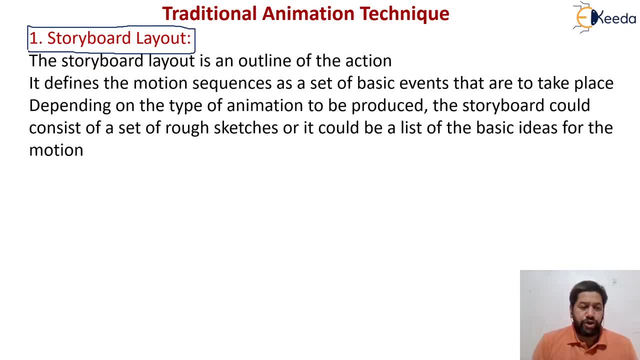 So let us understand what this indicate. Concentrate over here. The storyboard layout is an outline of the action in my step number one, I'm going to do, or I'm to go for the outline of my action. It defines. let us understand what it defines. 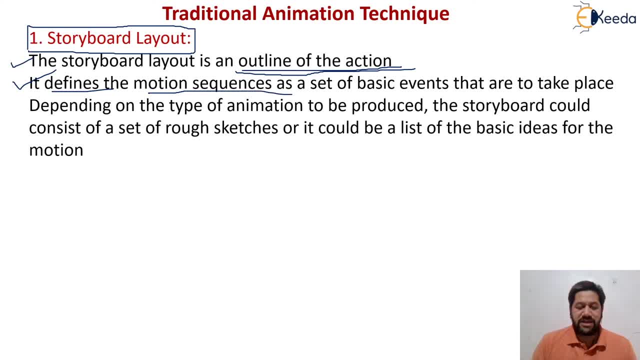 Okay, it defines the motion sequences. Okay, define the motion sequences as a set of basic event that are to take place. Okay, depending upon now, what it is going to define Basically is degree is going to define the motion sequences as a set of basic event that are going to take place. 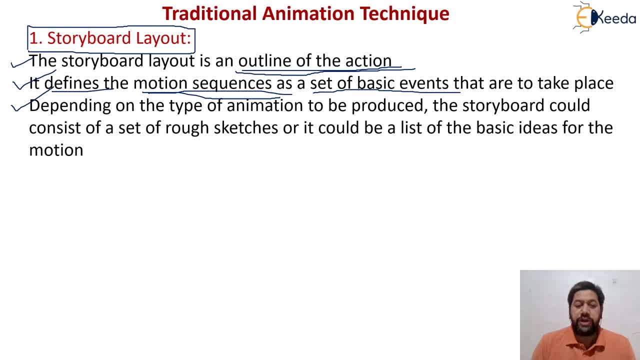 Okay Now, the next point I have mentioned is depending upon the type of animation. Okay, what type of animation I have to provide to? depending upon the type of animation To be produced? Okay, the storyboard would consist of a set of rough sketches. 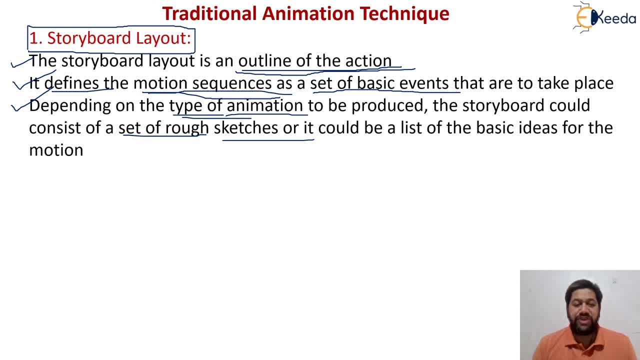 That's why I say to the layout: Okay, so I'm having to consist of a set of rough sketches, or it could be a list of basic ideas for the motion. Okay, so it may be the list of the basic ideas for the motion. 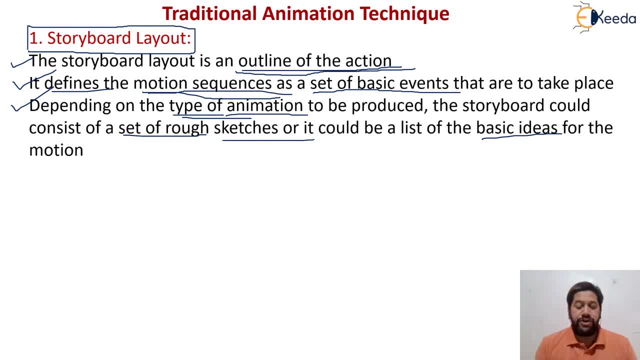 I think all of you are already knowing that if you are considering whatever the video that you are listening Now, this video is also having the n number of things are generated. I think nowadays, so many applications are available, So many apps are available. 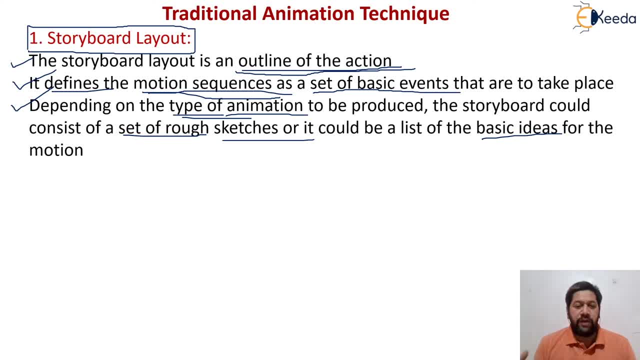 Okay, where you can modify or edit your video. Okay, And in that video you can find that it is made up of so many frames. You can delete some part of the video and so on. So all these things are possible for that. 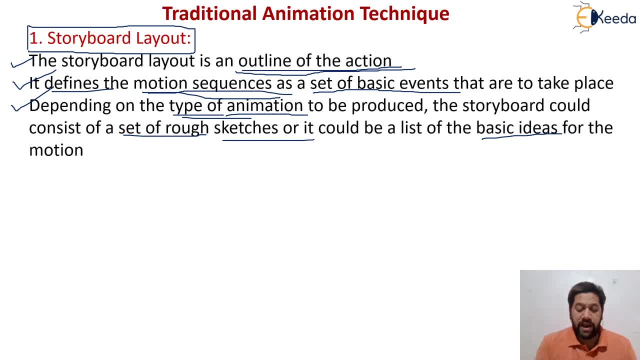 We have to mention where to go for the layout. Okay, and that is my storyboard layout that we have to consider. Okay, So that is what my step number one, that is known as storyboard layout. What is my step number two in my animation? see in my animation. 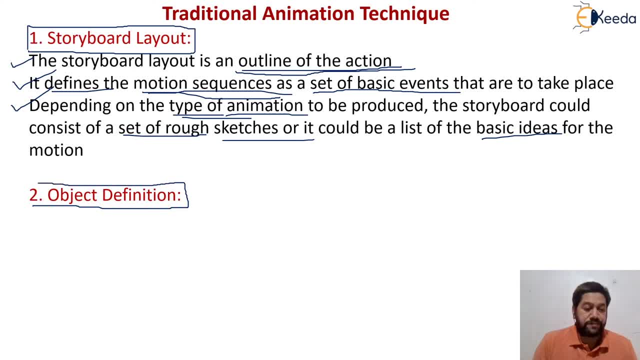 My step number two is observation. Object definition: Okay, after the storyboard layout is over, My second step is object definition. Okay, that I'm going to follow, or that is, I'm going to use it as an object definition. So what is mean by object definition? 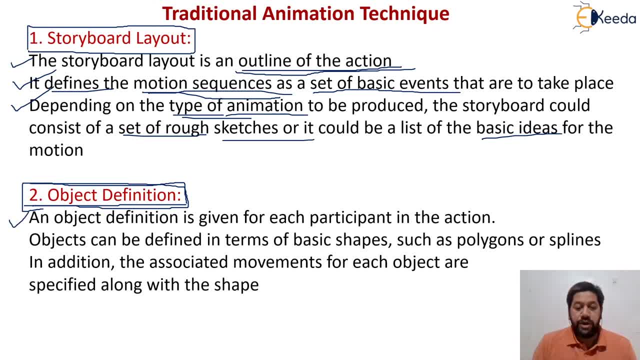 He. an object definition is a given for each participant in the action. So in my action I have to find out how many objects are involved- Okay, how many objects are there? and I have to define all the objects. Okay, I'm just considering it as the example. 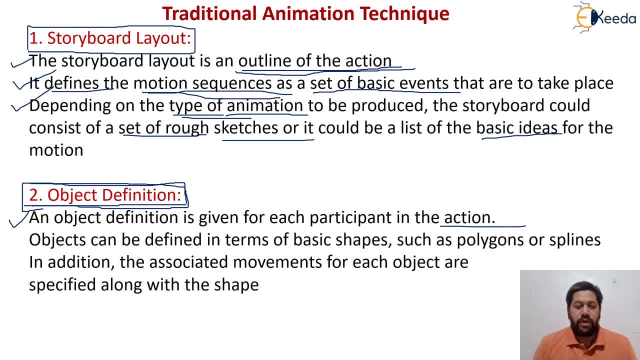 For example, those who are watching to the Chhota beam as a cartoon or any cartoon you can find. So, first thing that they decide which are the objects. are there? Okay, maybe Bheem is one of the object. Okay, I think another. I think, as I remember, in the Chutki is another object. 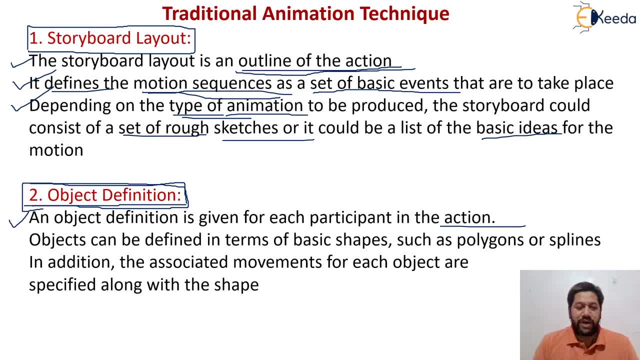 Okay, we are having the Golubolu is another object. We are having some monkeys there in that case. So first we have to define how many objects are participate in that action. Okay, if they are showing that another person is there in that cartoon or that movie who is considered as the villain, who is playing the role of the villain or any other thing. 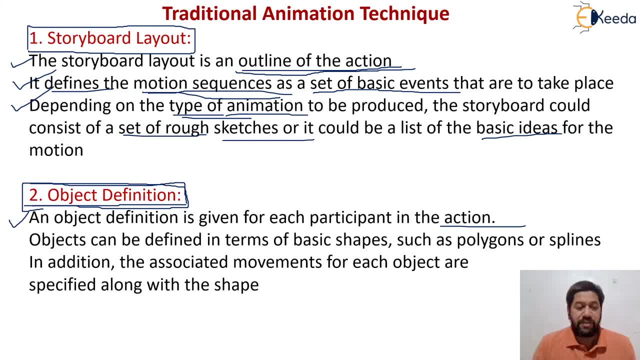 So that object should be defined. Okay, So here, what we have to define is step number two. We have to define the object, which is called as an object. definition is given for each participant in the action. Okay, Next, what we are going to do. objects can be defined in terms of the basic shape. 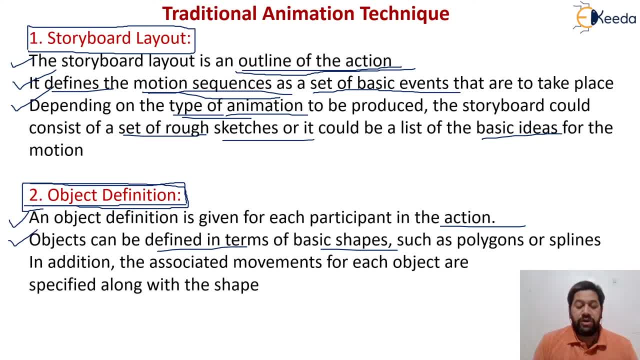 So we have to decide. suppose I take the example of Bheem. We have to decide: What is the shape of that particular object? Okay, how it is represented with the polygons and maybe the spline. Okay, so different curves are there, that we have to use the different polygons. 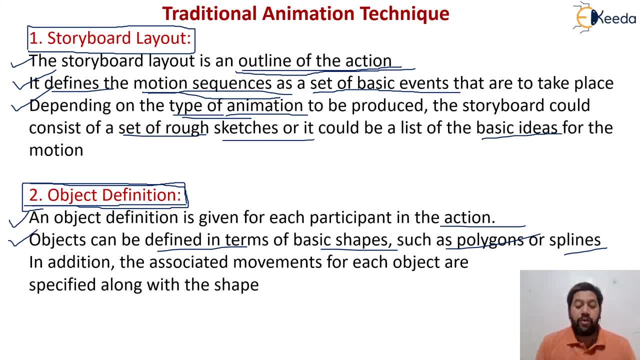 We have to decide the color of that particular object. Okay, I think nowadays- that's why I told nowadays- the animation industry has reached at the level that they also define the same object. Maybe suppose I consider the Chota Bheem Bheem is one of the object that will show that how that object will look like whenever it is laughing, how that object will look like whenever it is surprised. 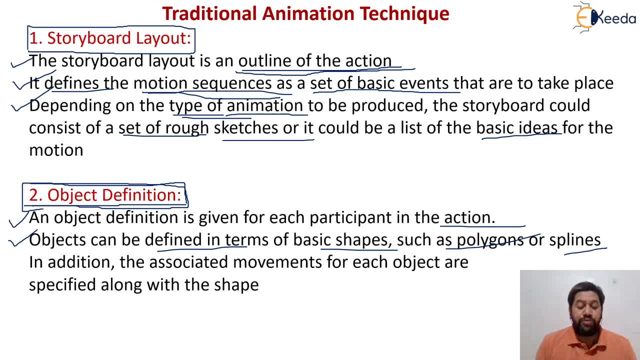 When, how that object will look like whenever it is crying, how the object will look like whenever that object is angry. Okay, so all this definition that we have to define, Okay, we have to define that- how that object look like, and that is what we call it as the object definition. 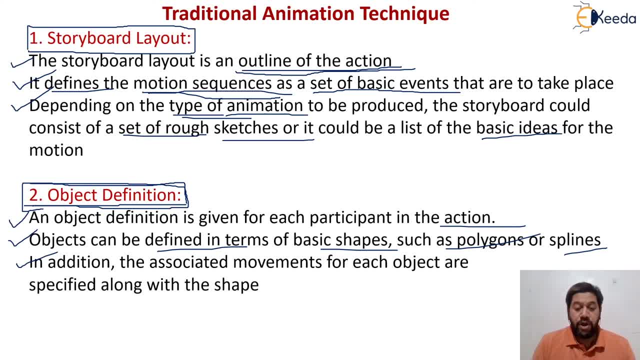 Okay, so in addition to the associated moment for each object, are specified along the ship. Okay, because that shape is going to define. see, suppose that particular object is running. if the object is jumping, Okay, How will it will look like. so for all these things, or all these moments of that particular object. 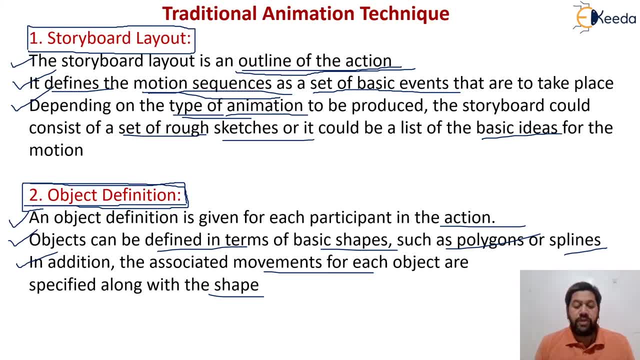 Okay, maybe it is running, maybe jumping, Maybe it is sitting down, Maybe it is standing to whatever that we have decided, we have to define this object definition. That is why I call it as my step number one for the step number two. step number one is storyboard layout. 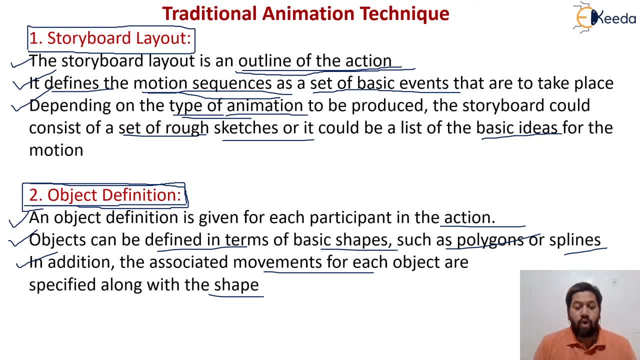 Then we have to go for the object definition. So we have to find all the objects who are going to participate in that action. Okay, it is available in that particular, Maybe the video for particular frame that we have to define. Okay, so this is my step number two in my animation technique. 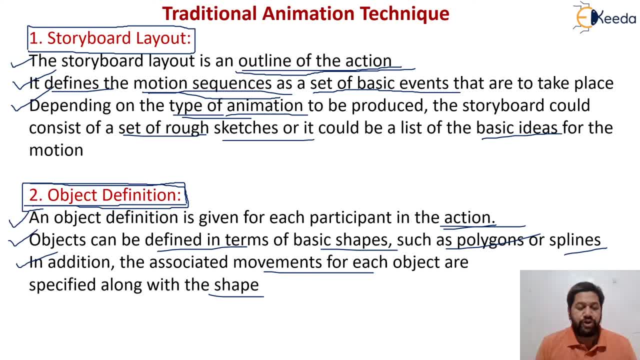 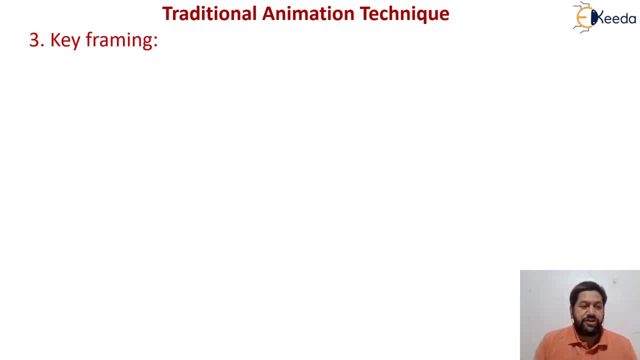 Okay, let us understand What is my step number three now. Okay, I'm just moving now to step number three. to understand the next step. Okay, see, this is my step. number three is having the name, or it is known as the key framing. 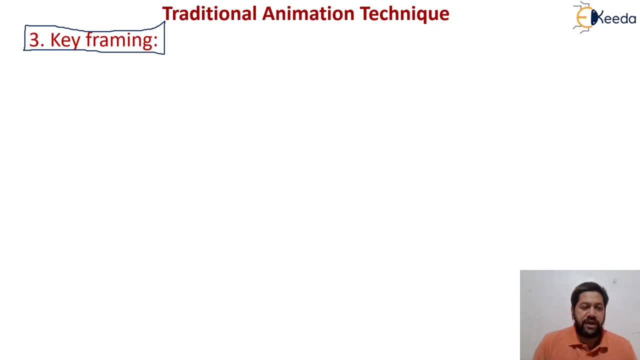 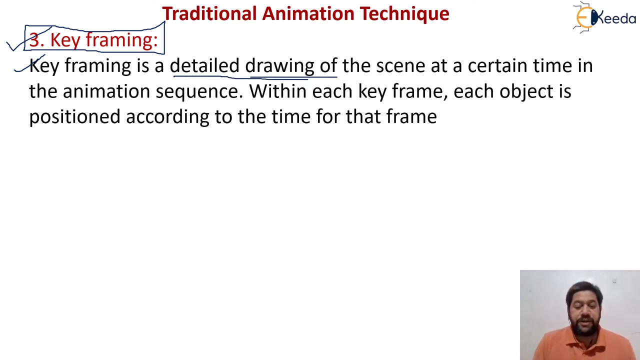 Okay, what is my step? number three in my animation technique is- it is number three- key framing. Now, what is mean by the key framing? So, key framing, the first point, key framing is a detailed drawing. see here. Now I am having detailed drawing, the first step, what I have done. 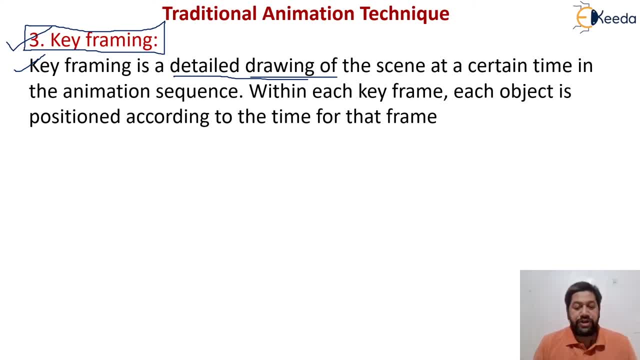 I have done the outline. Okay, I have done the outline of that particular sketch. Okay, what is the outline here? number two: I have defined that object in object. Now, what I am doing in three framing, it is detailed drawing of a scene at a certain time in animation sequence. 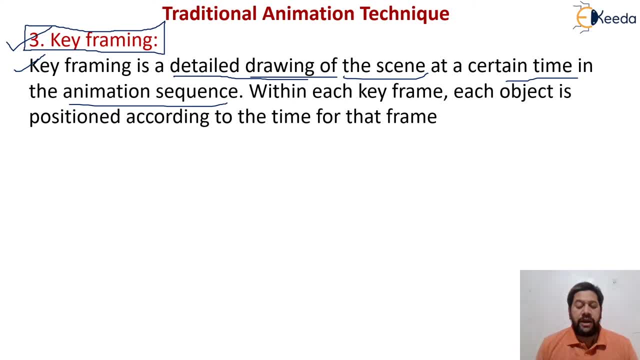 Okay, So means at time, suppose I have started animation. What should be there? What should be the scene in first minute? second minute, What is the scene third minute? What is the scene where the same scene is continued for next time? So all this will be detailed. detailed drawing of the scene will help for go for the framing. 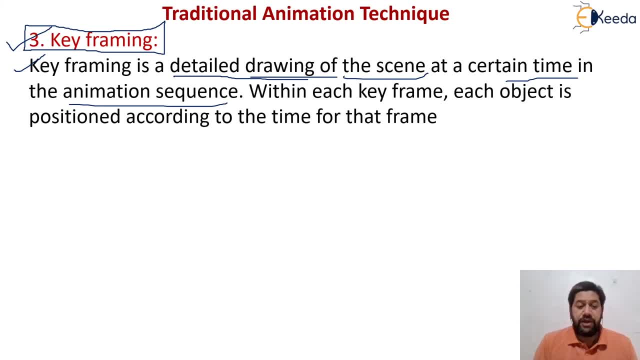 Okay, read again what I have written. key framing is a detailed drawing of a scene at certain time in the animation sequence. Within each key frame, Each object is position according to the time for that frame. Okay, each object is position according to the time for that frame. 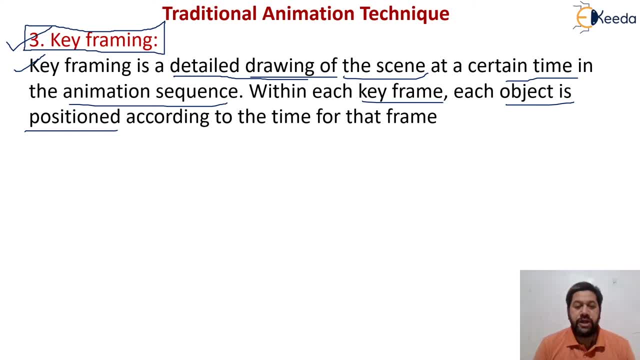 See, for example, at this particular moment of the animation: Okay, I know that this object is at central place. another object at the left side place, third object, will not be displayed over there. We have to say that at each frame which objects we are going to display and what is the position of those object. 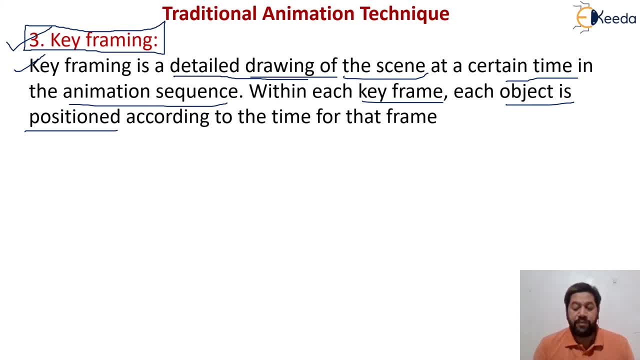 Okay, where this will be position with respect to the time Of that particular frame and that we are doing in the key framing. now let us understand the second point. some key frames are chosen as extreme positions in the action. Okay, that may be extreme position in the action, others are faced. 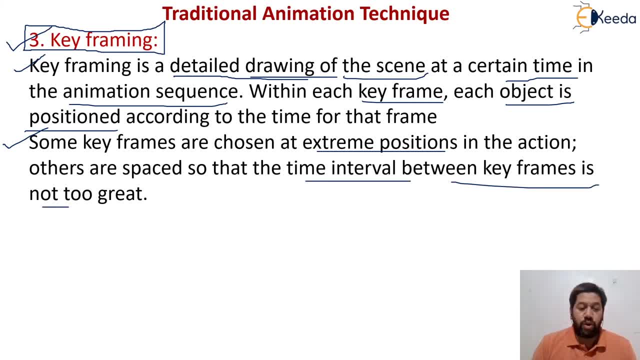 So that the time interval between the key frame is not to breath. Okay, See, some key frames are chosen at extreme position in the action. indicate that other are. space means other objects of space, so that the time interval between the key frame is not too great. 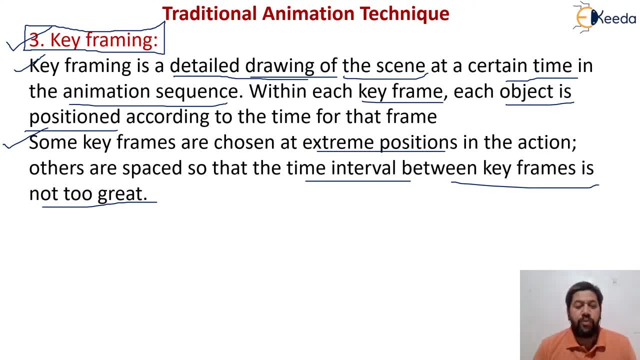 to great, which will be maximum T same. only some of the objects are moving here and there. Okay, so maximum time the main object is will be focused. It will be at the center place. So that is what we are considering in this particular case. 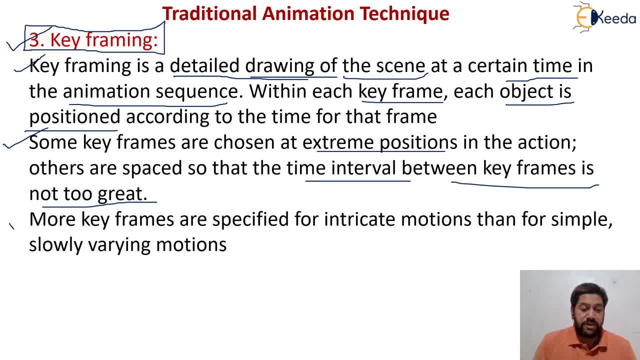 Okay, Now let us continue discussion. more key frames are specified for intricate the motion. Okay, to indicate the motion for simple and slowly wearing motion. So I have to add some more key frames. Suppose I want that my motion to be very slow or it is simple. 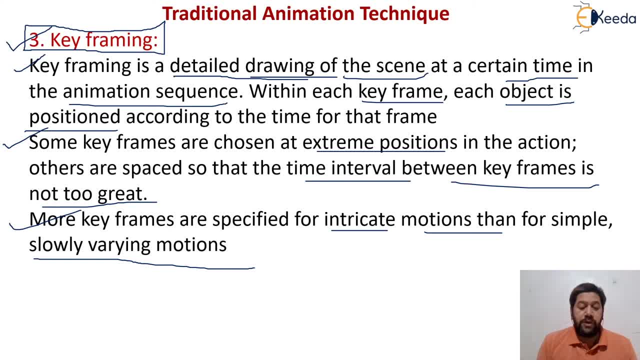 or it is slowly wearing, slowly moving from having the motion to be slowly wearing, then I have to add more keyframes. additional keyframes I have to add into that so that it I can show that it is moving. Okay, so additional frames I am going to add into this. 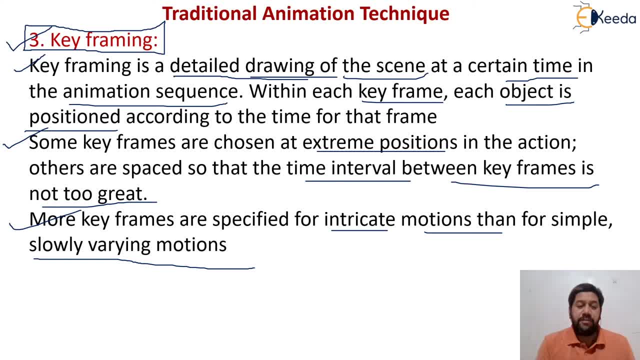 and that is part of my key framing. See, we are going to learn this key framing in one of the session in detail. Okay, so that we call it as a key framing system that we are going to learn all the details of related to the key framing. but just understand now. 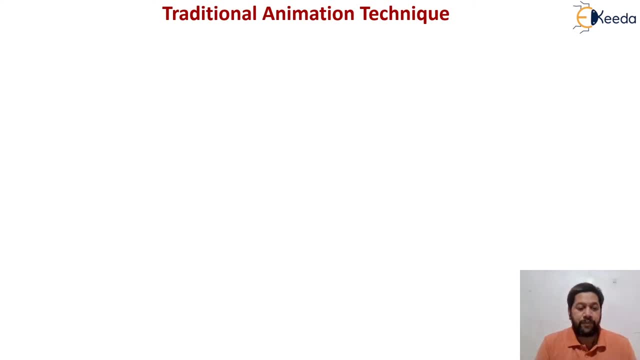 This is my step number three. in my animation is key framing. Okay, Now, what is my step number four now? So this is my step number four, or the last step that we call it as in my animation technique. What is this step? 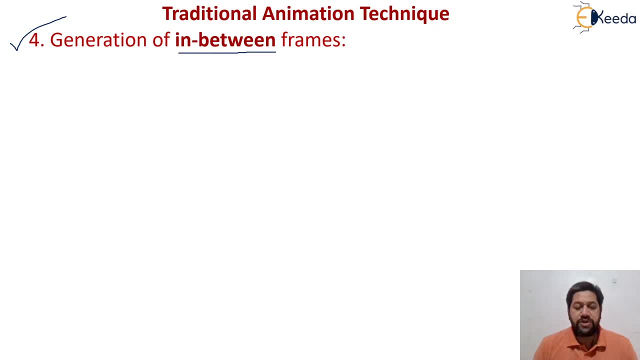 It is called as generation of in-between frames. Okay, keep framing. Now we are having generation of in-between frames already. simply all that in-between frames. Okay, so I have to generate the in-between frames which are matching my every frame In-between. 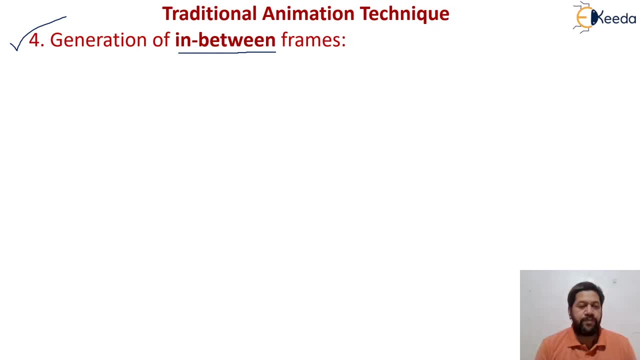 Okay, so that I have to do, or that I have to consider. Okay, let us understand. what is this Now? in between, what is mean by in-between? So in-betweens are intermediate frames between the key frames. I'm having, this is the key frame and in between, the key frame. 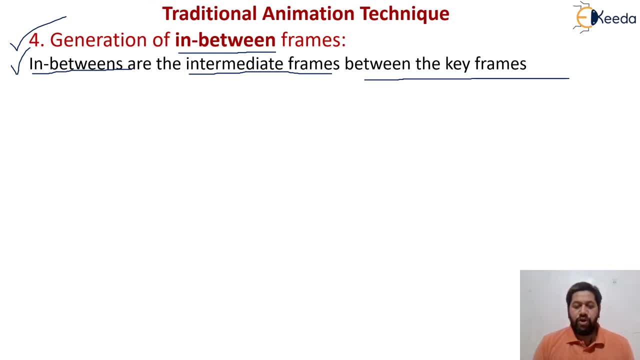 I am having the intermediate frame. Okay, so I'm having the initially as a key frame in key frame, in between and required, so that's why the name is given as in-betweens are the intermediate frame that I am going to add between my key frames. 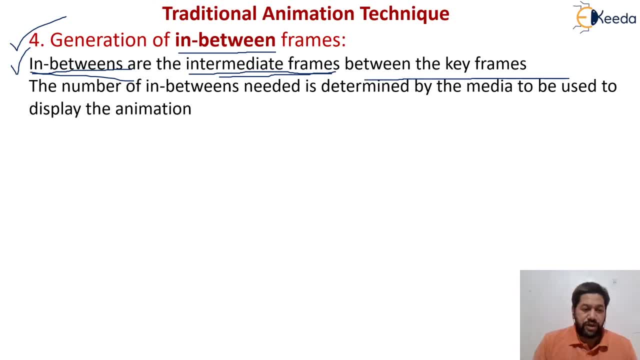 Okay, Now the number of in-between frames. So next thing is very important: the number of in-between frames needed, How many frames are required in between. So number of in-between frames are needed, How many I've required in between frames, is determined. 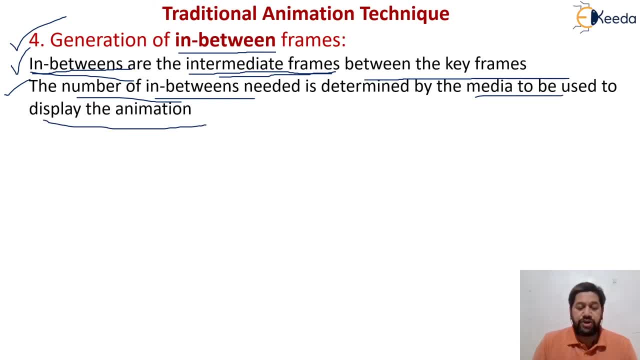 by the media to be used to display the animation, What media I'm using, how I'm going to display that will matter that. how many in-between frames I'm going to use, Okay Now, for example. that's why I am saying, for the film requires. 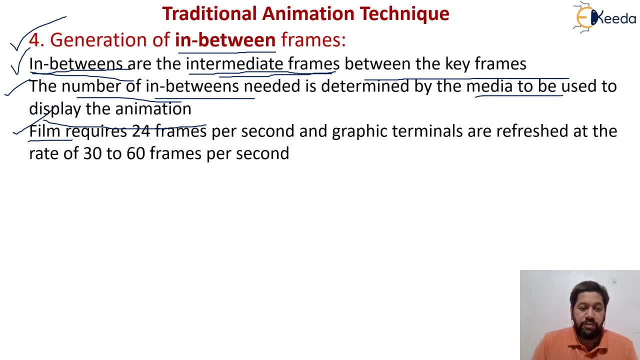 the was. I'm considering it as a film, animated film, So film generally requires 24 frames per second. Okay, for per second I have to ready my 24 frame. So you will ask whether all these 24 frames are of different type. 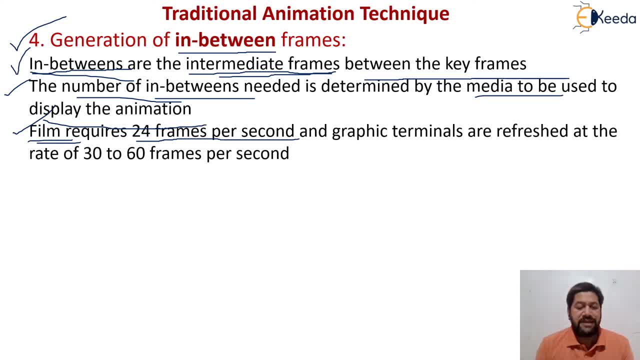 No out of 24.. Maybe my key frames are only 5, 6, 7.. Okay, and in between I'm adding my in-between frame. So that is what the point of discussion. Okay, so I'm adding in-between frames here. 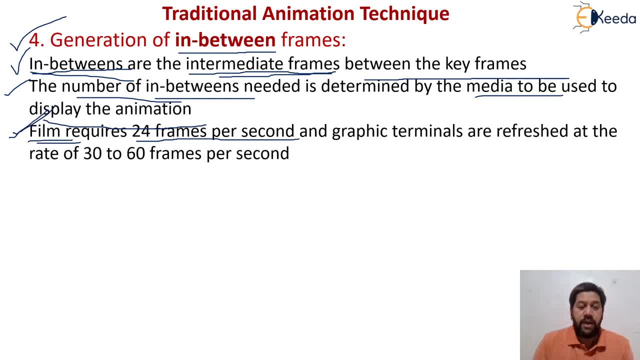 So if I'm in considering film industry or for the film, I required 24 frames per second. If I'm displaying on the graphics terminal or refresh at the I all of your knowing, Okay, we have learned that there is a graphic refresh cycle. 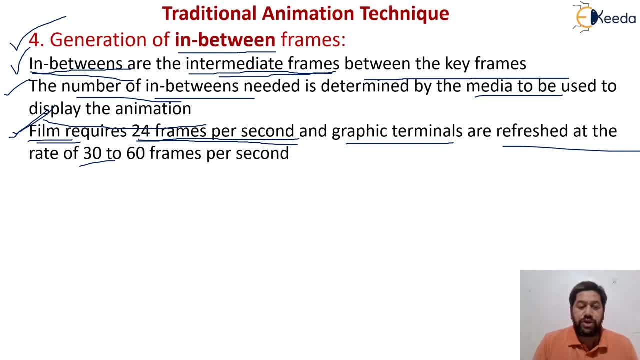 So that refresh at the graphic required the rate of 30 to 60 frames per second. Okay, it's actually film required 24, but the graphics required 30 to 60 frames per second. So definitely I have to add the in-between frames. 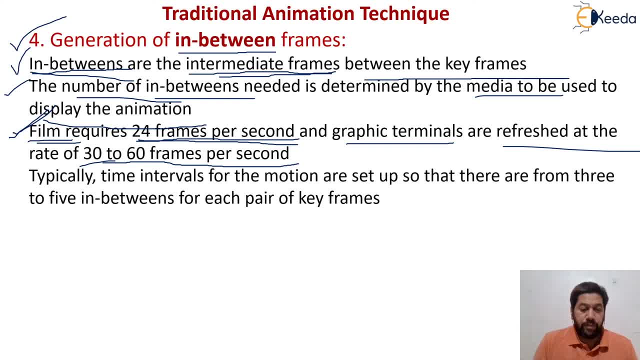 Okay, so no choice. We have to add in between frames. generally, or typically, the time interval for the motion are set up. Okay, time intervals for the motion picture are set up so that there are from 3 to 5 in between. That's why that is what I told. there may be minimum 3. 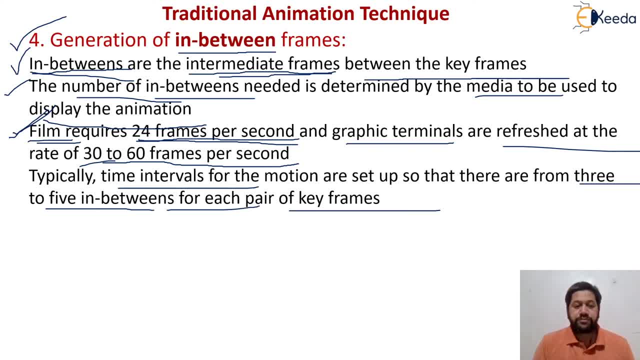 to 5 in between for each pair of keyframes. Okay, see, I'm having the first keyframe, then my second keyframe. So in between my first and second keyframe, generally there will be minimum 3 in between frames or 5 in between frames between this pair that we have to add. 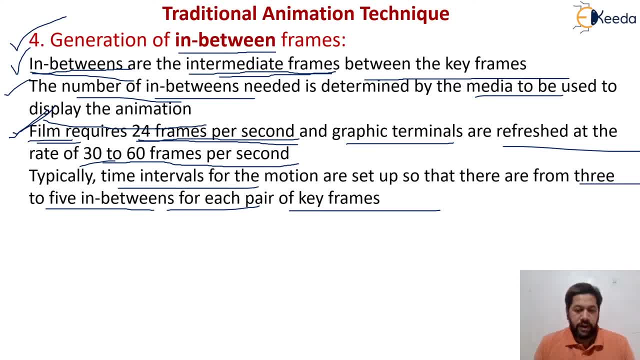 so that I will look at that. It will be moving, will be motion. Okay, so that's we are considering. Now I just continue our discussion that I'm giving some example over here. See, this example will definitely help you. That's why I say why. it is helpful means it will understand. 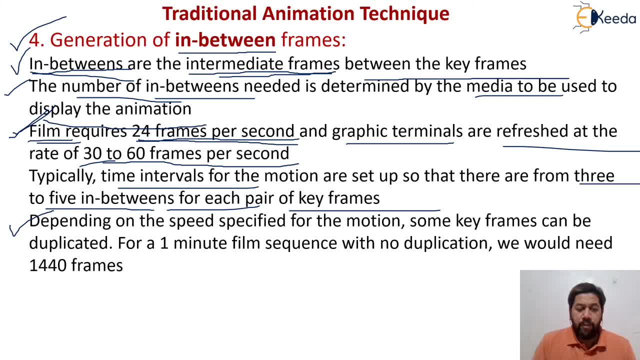 how exactly the in-between frames are used. Okay, so, depending upon this Speed specified for the motion, So how much speed you want for that motion- some keyframes can be duplicated. Okay, so some keyframes I'm going to duplicate, depending upon. 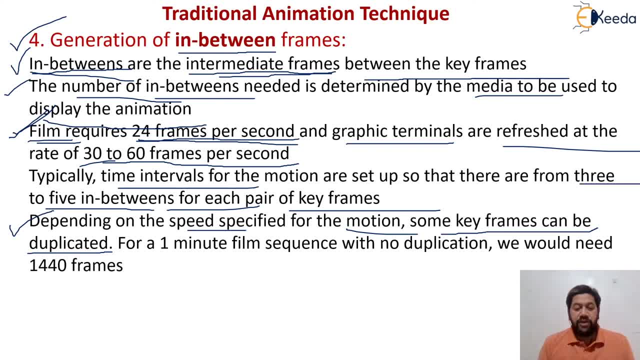 how much speed I want. So first you define what is the keyframe and then it is required depending upon the motion. if the motion is very slow, Okay, the object is moving very slowly. So I need to add the duplicate frames also to the keyframes can be duplicated. 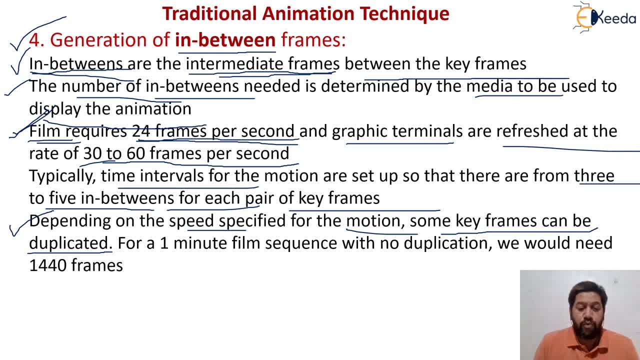 Okay, you will surprise if I just give this as an example For one minute film. Okay, I want to record, or I have our animation of only one minute film sequence, with no duplicate. I'm not letting you bring. we would need around 1440.. 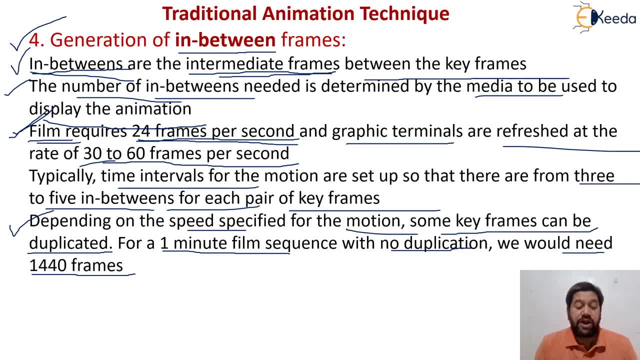 Okay, I think 1440 frames are required for a one minute video. Okay, then you can observe and you can understand why there is need for the in-between frame. So, whether I'm having this 1440 frames, all are my keyframes. 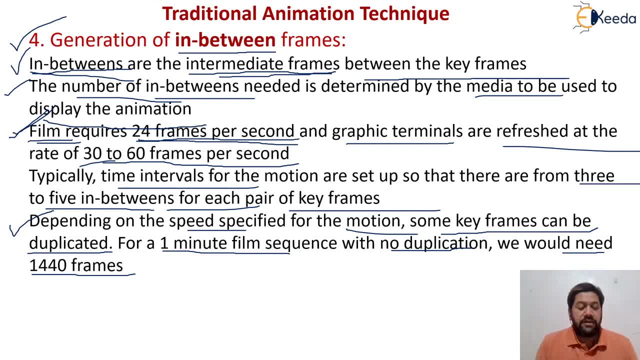 Definitely It is not possible. Okay, so I'm having very less keyframes in between. I have to add to that where the name is given as in-between frame: generation of in-between, in-between frames. I need to generate, I need to add all these in-between frames. 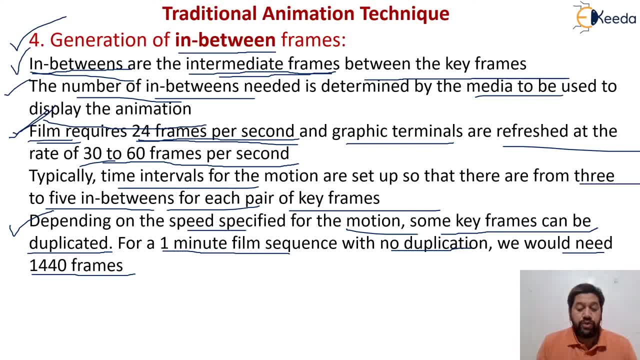 Okay in my film or in my animated video, so that I will get it Okay, because definitely it is not possible to have 1440 keyframes or original frames. Okay, so that is, that is not possible. So that's why there is need to go for in-between frames. 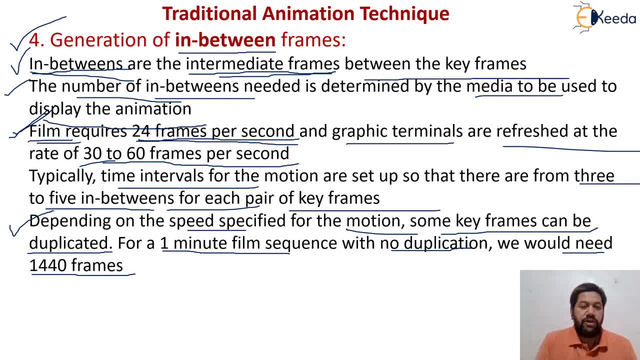 Okay, I continue this example. Okay, so that you will understand the importance of the in-between frames. Now I say that with how you in between. suppose I'm using how you in between between a pair, Okay, between two keyframes. I am using how you in between frames. 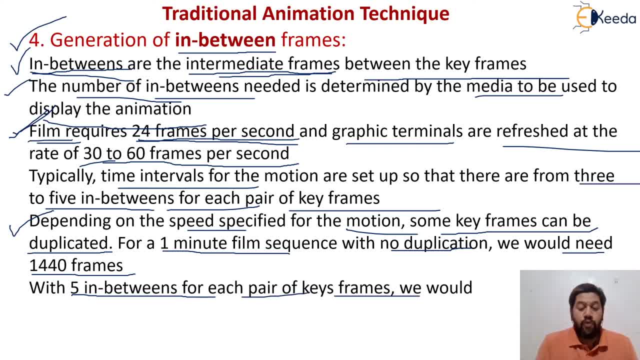 Okay, for each pair of the keyframes. Okay, how much I will get? we will need 288 keyframes. Okay, see, I just explained it again so that you will understand. for a one-minute field, Okay, for one-minute film, I think we are having here required minimum 24 frames per second. 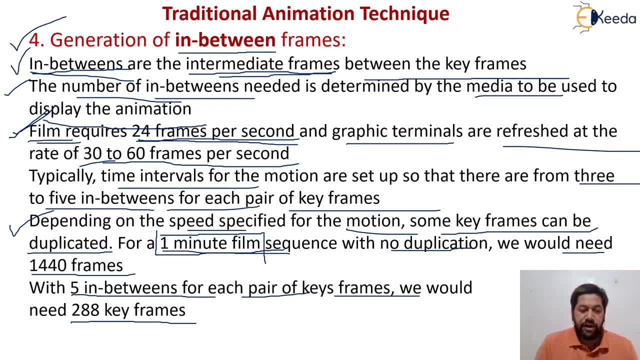 Okay, 24 frames per second into 60.. I think I will get here about 1440 frames are required. Okay, and out of this 1440 frame, suppose I have decided to use how you in between frames, between the two keyframes. 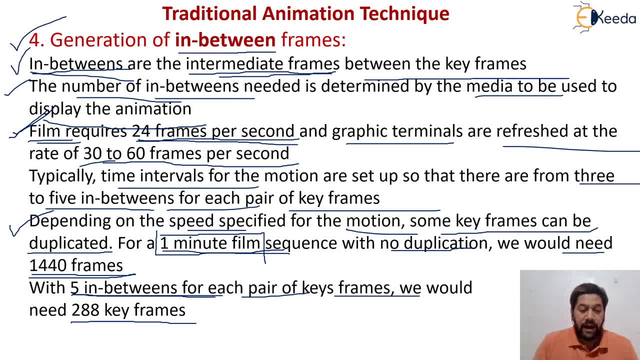 You have used how you, I think. then also, I required around 288 keyframes are required just to generate 288. Main frames: 288 keyframes are required just to produce the animation film of one minute. Okay, so that's why you will understand how much difficulty. 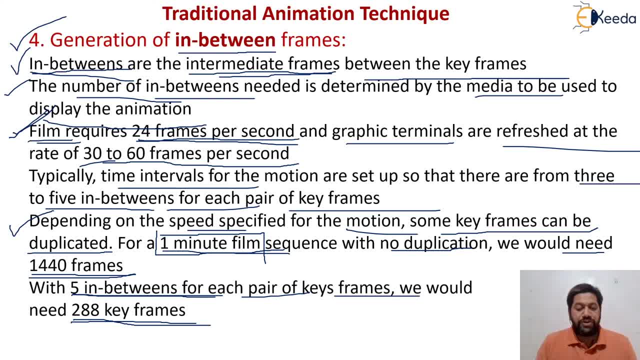 is just record for the 15 minutes, 30 minutes. How much time is required? How much work is involved in that case? Okay, So this is what you're having related to the generation of the in-between frames. Okay, I hope all of you understood. 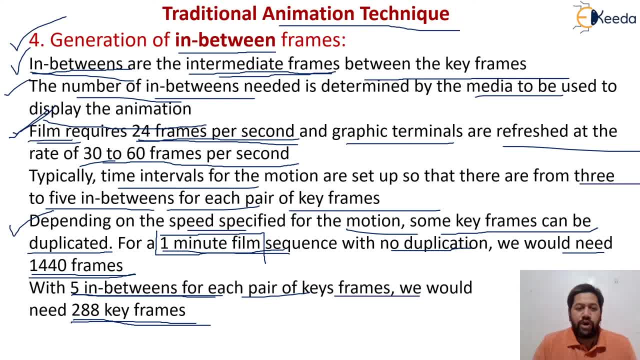 This is my animation technique. I do call it as a traditional animation technique Because it is initially designed by considering the cartoon animation or animation of the cartoon, but it is applicable to everywhere, in every application. It is applicable, maybe with some modification, Okay, so which I repeat again. 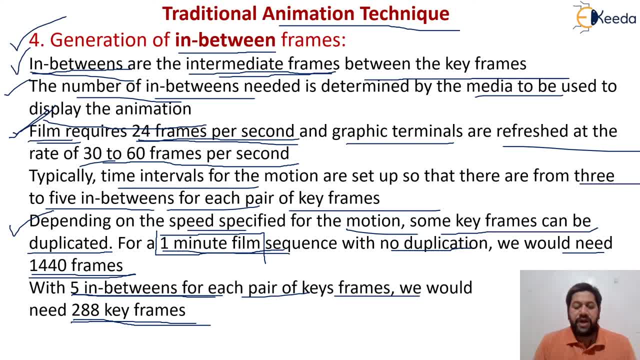 which are these four steps that we are having? the first step, We are considering it as the storyboard layout. Okay, step number one is storyboard layout. step Number two is we call it as the object definition. The third step is key framing and the fourth step is generation of the in-between frames. 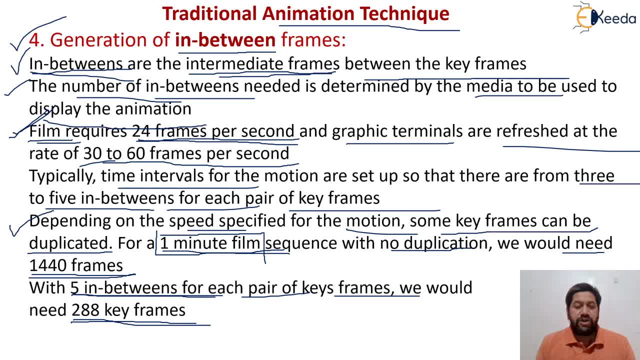 Okay, getting me. So this is what the four steps are there, or these four tips are involved in the animation technique. If I want to generate any animation, I have to follow these four steps there and then only it is possible for me to get into the details. 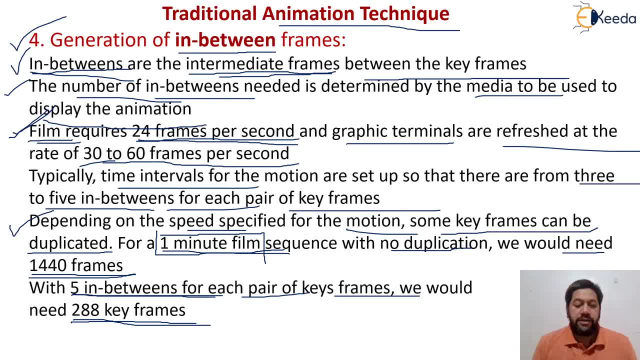 Okay, so with this background, or with this understanding, now I'm just going to show you some diagram, or with the example, so that you will understand this particular point in detail, will understand that, how I am going to Use this animation technique or how the animated images will look like. 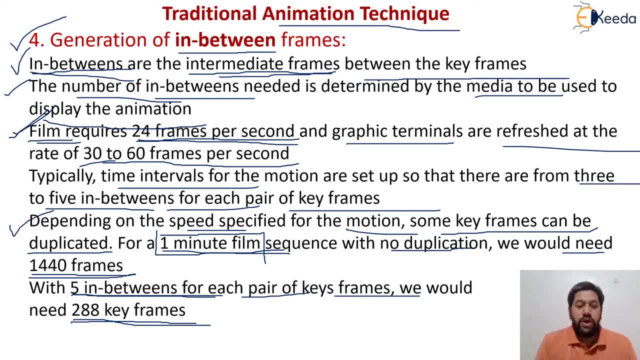 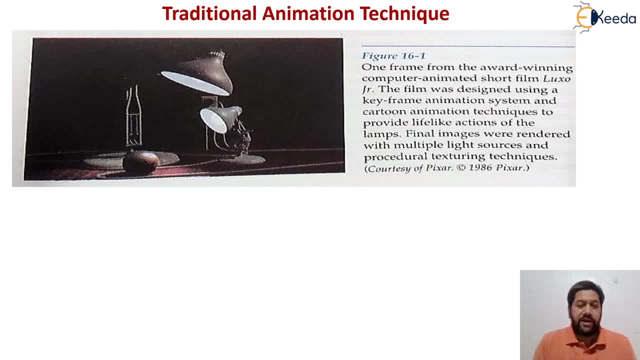 Okay, that's why I'm just moving to the next slide, to show you the different examples related to the animation. Okay, So here you can find the diagram, as you have shown this as my diagram number one. Okay, So this is what we can show. 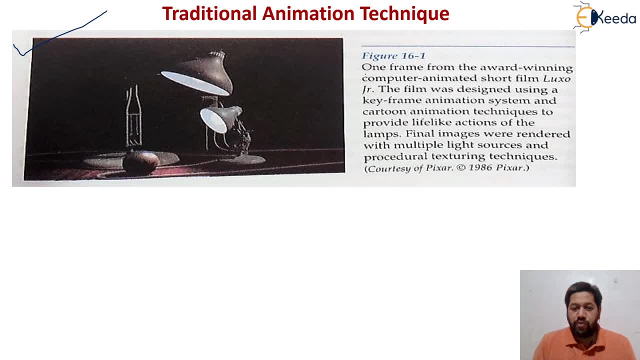 This is what the animation that we are having. Okay, so I'm just showing you one frame from the award-winning computer animated short film Look so LUXO. Okay, so, from this film, I'm just showing you the one frame. 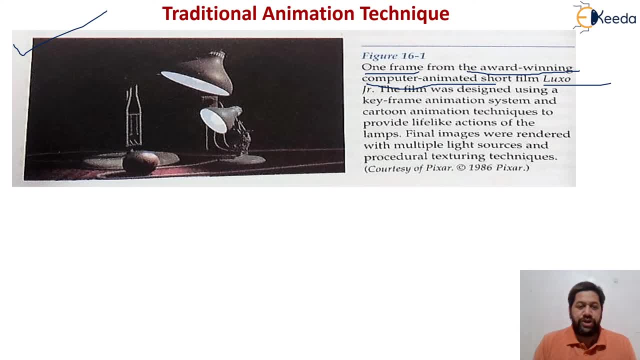 Okay, this is the award-winning short film. is there? animated short film was there, and now this is one of the frame of that particular object. in this frame You can find: this is okay, This may be the realistic object, but this and this may be the computer generated object. 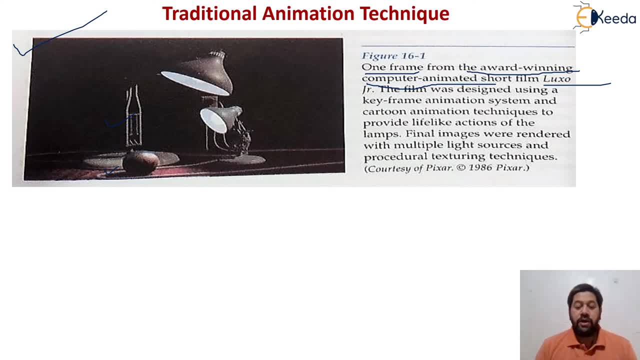 We are showing. we are showing the effect there. visual effects are there. Okay, so so many things are involved in just developing this frame. Okay, the film was designed Using a key frame animation system and cartoon animation technique to provide the lifelike actions of the lamps. 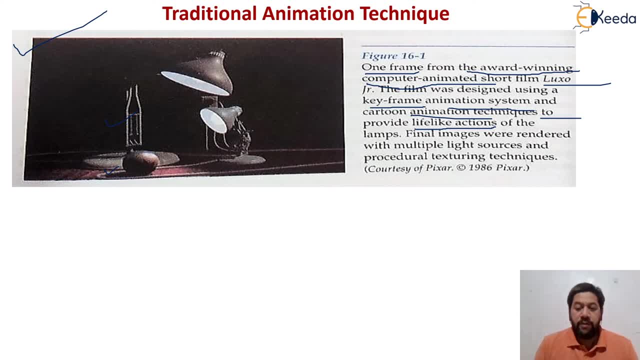 Okay, it is going to show the lifelike actions of the lamps. Okay, final images were rendered with the multiple light sources and procedural texturing techniques. Okay, and this is what one of the frame or one of the image of the award-winning computer animated short film called as the LUXO. 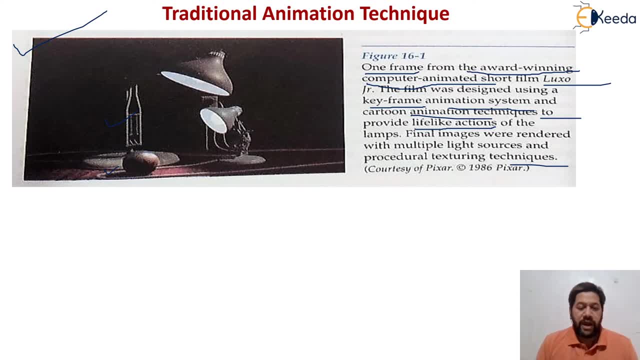 Okay, and that is what we have shown. Okay, generally, I think we are more interested into the different cartoons. Okay, the cartoon frame is there, So that's why I'm showing you the next example where we are going to look: a cartoon generated image. 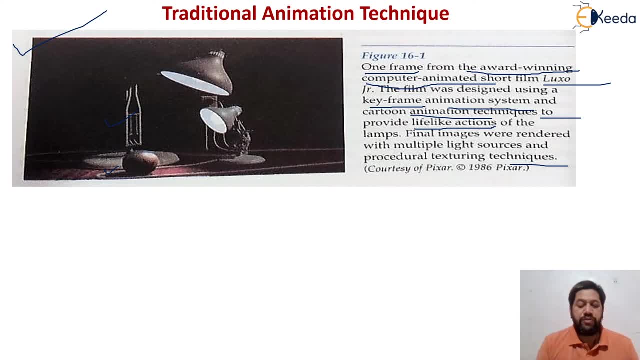 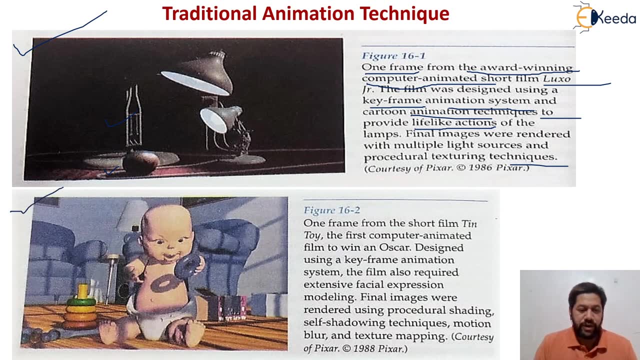 Okay, so that is what the example or that we are generate with the help of the animation. Okay, so let us understand this Now, here you can find it. here You can find this particular example number two: Okay, So one frame from the short film: teen toy. 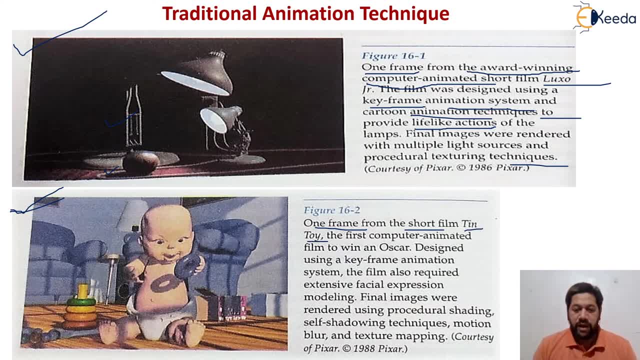 Okay, teen toy is one of the cartoon film that we are having. Okay, This is the first computer animated film to win an Oscar. Okay, So remember, this is the frame which is shown over here. This has okay, and the name of the short film is teen toy. 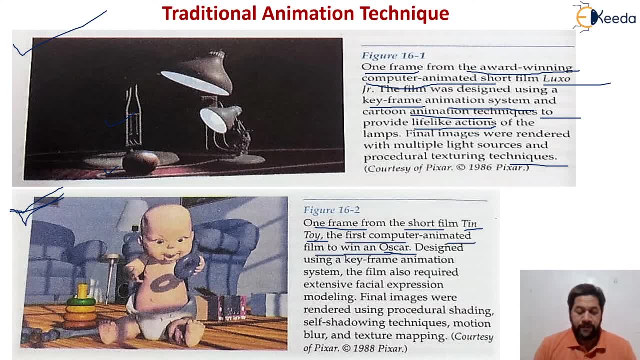 The first computer animated film to win Oscar. Okay, This is also designed using the key frame animation system. The film also required extensive You facial expression. I think I have discussed just now. Okay, What I told is: I told that there is a facial expression is required. 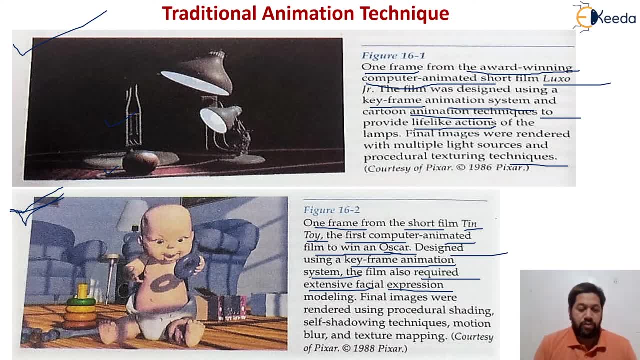 That is what I told. whenever we are defining the object, When I deploy- suppose I consider this is my object. Okay, What is my main character on my main object? This is my main object, Okay. So whenever I am defining this main object, 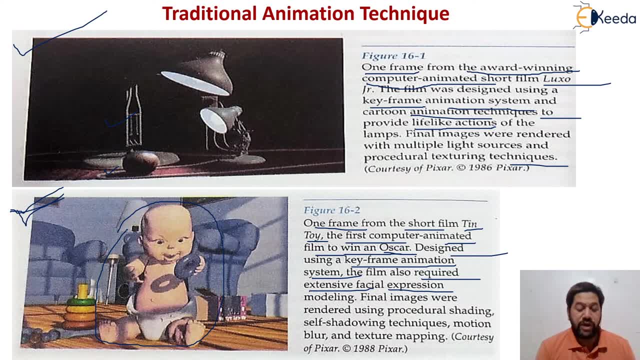 I also have to define the facial expression. Okay, so you can find that here. that particular object is surprise. Okay, It is giving some reaction. So that is what I told. we have to define that: how the object will look like whenever the object is angry. how the object will look like whenever the object 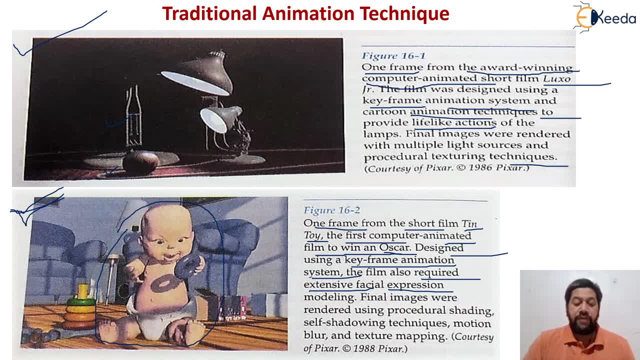 is crying, Okay, how the animated object will look like whenever it is. Yeah, I see it as Kate is angry, or maybe surprise, maybe laughing, Okay, So all these things are there. So that's why I just required the facial expression. 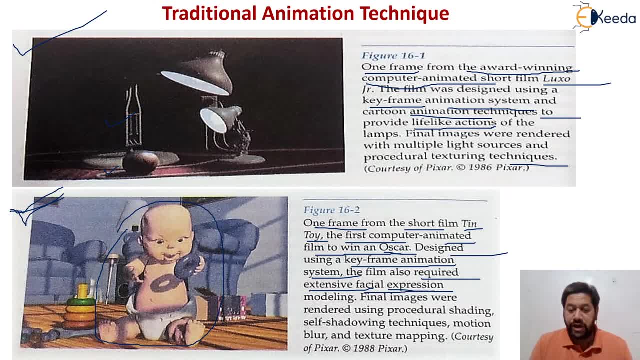 Okay, So the film also required the extensive facial expression modeling is required. Okay, final images were rendered using the procedural shading, self-shadowing techniques and so on. Okay, you can find. this is the one of the object. another object You can find here: 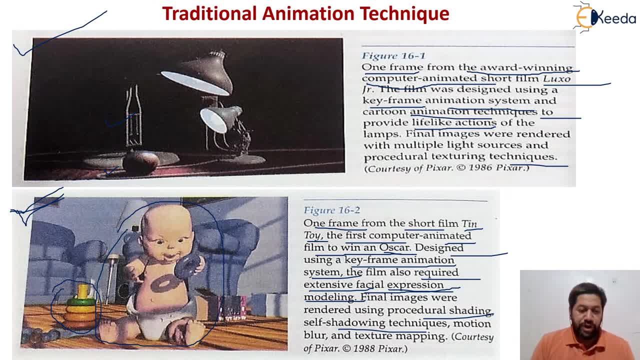 This is another object. Okay, Now this is going to put it over here, suppose. Okay, So the animation or the motion is required in this particular case. You can find at the background We are having. this is the background image is also there. 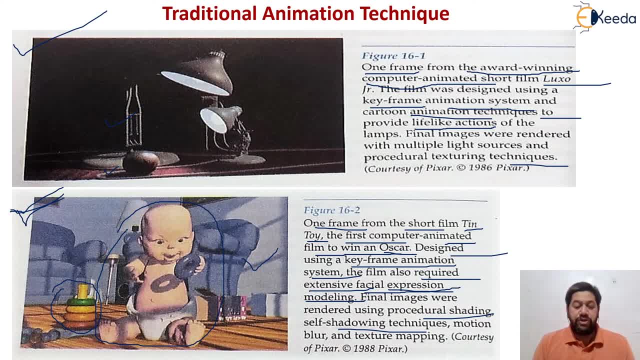 Okay, So all this thing should be generated with the help of the animation. Okay, So that's why I say that This animation is one of the, though It is a part of computer graphics. I call it, as it is, a separate subject of the interest or the separate subject of the research. 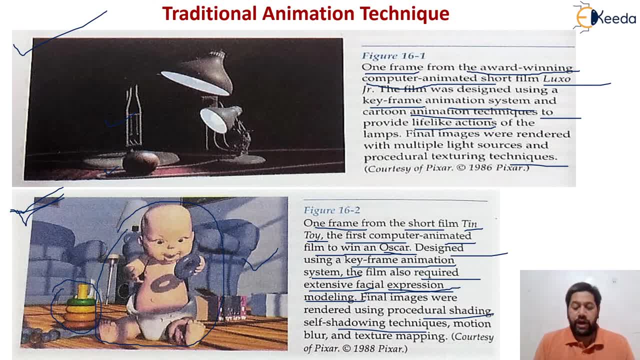 Okay, where we are going to go for the learning the animation technique in detail. Okay, We are just learning This is one of the sub part of the computer graphics, So we are just learning the very basic things of the animation Okay. 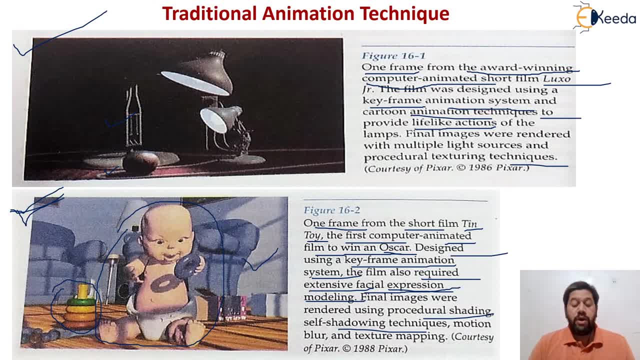 Now I'm just showing on the next slide: Okay, So in animation, What we need to do, see, we have, long already, the rotation: Okay, we have learned two-dimensional rotation. We have learned the three-dimensional rotation- Okay, but I want that this object should be rotated. 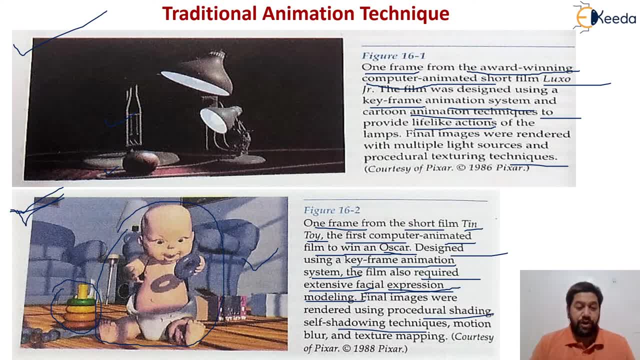 This object should be moved- Okay, not only this particular object, but I think it is necessary that. so I'm just showing what the one example is. the next slide to understand that how this 360-degree rotation is required, and not only for the one object part, but it's required for all the parts of the object. 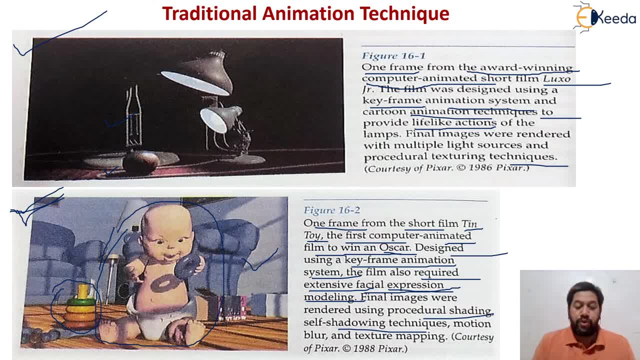 Okay, For example, I'm saying, was I take the same example of this particular, Okay, little boy with your, this particular object? I think I may require. it depends. I'm just saying you may require that the head should be rotated, Maybe 180 degree, 90 degree. 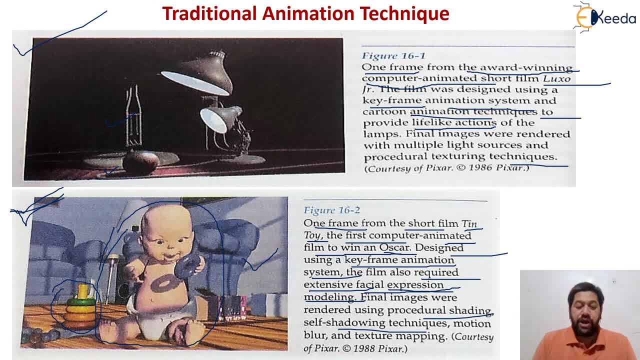 Okay, his legs or should be rotated in 180 degree, hand should be rotated in 360 degree, The complete object may be rotated into the 360 degree, and so on. Okay, So all these are the possibilities that we have to consider in the enemy. 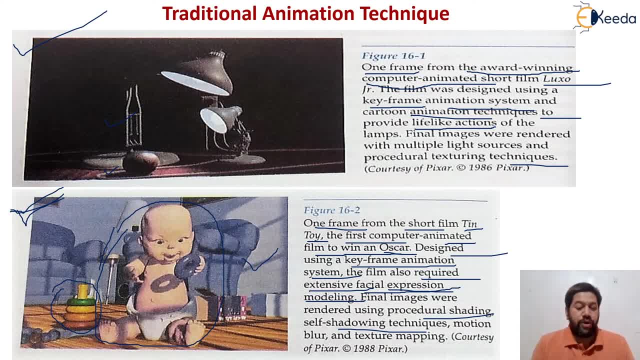 Okay, So these are the two examples. I'm just moving to one more example, or the slide that will help you to understand that for this animation is important and what we have to do. Okay, I'm just moving to the last slide, just to consider one more example of the animation. 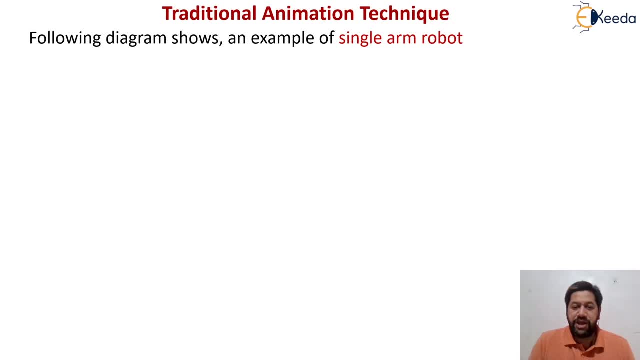 Okay. So this following diagram shows an example of a single arm robot. See, you know that if I'm going to design the robot, definitely the animation is required. without animation is not at all possible. Okay, Okay, to show that from here in this animation. for enough shoulder. 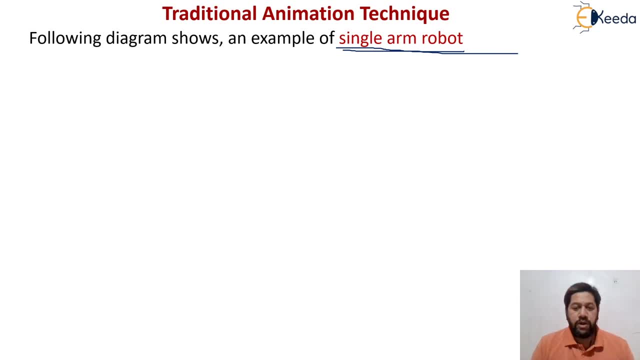 It is a single arm. It is showing there is only one arm of the robot. Okay, but the arm of the robot having so many parts and I want that all this part should be rotated, Okay, So that is what I'm considering. 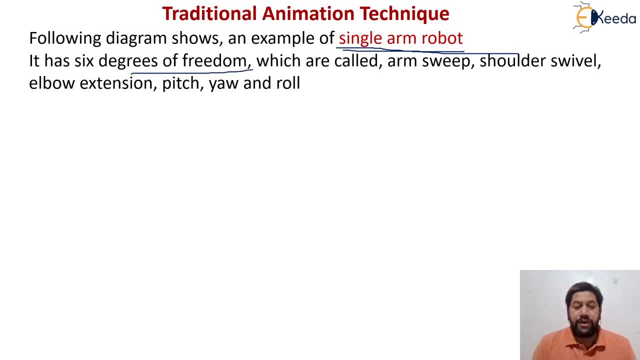 It had six degrees of the freedom. see degrees of the freedom indicate that the part can be rotated 360 degree. I want you should be rotated 360 degree. which are called on? which are these parts and I'm having? Okay, It is the arms with a shoulder. 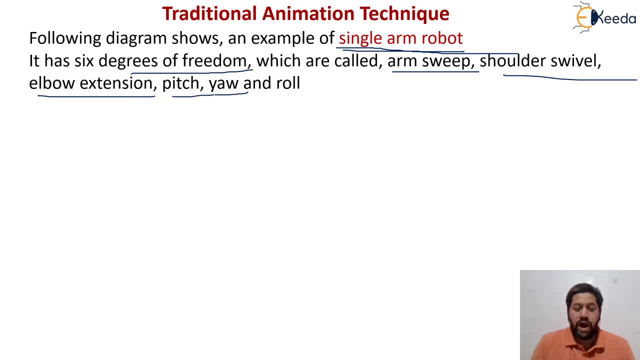 We will Elbow extension, pitch your and roll and so on. So so many parts are there and I want that all this should be rotated into the 360 degree and that is called as a degree of freedom. Okay, for that particular object, for that particular animated object that I am considering. 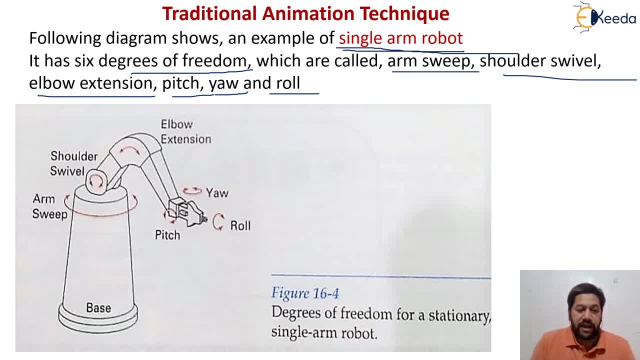 Okay, let us understand the diagram. Yes, you can look at this particular diagram. see here I have written What is the name of the diagram. is degree of freedom for a stationary single arm robot. Okay, single arm robot, I want degree of freedom here. 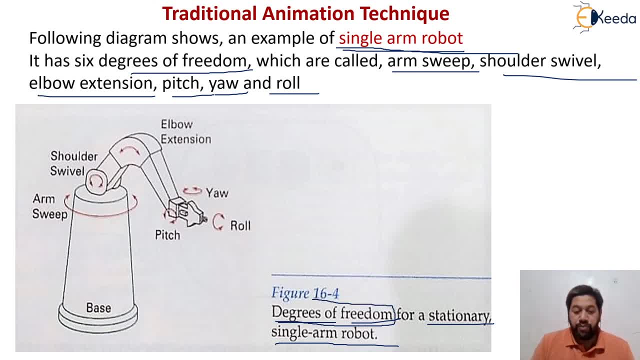 What is mean by degrees of freedom indicate that I should in the position to rotate that object in 360 degree. Okay, I can perform the rotation. in 360 degree means I will get the degree of freedom. Okay, Now you can find here this particular arm. 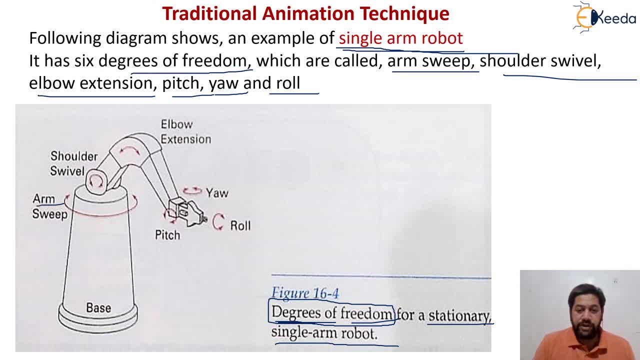 You can find this arm itself. Okay, that I am calling it as the arm slip. Okay, this arm is also rotated. You can find this will be rotated. Okay, this is the shoulder of that particular robot. should be rotated this shoulder. Okay, suppose I consider this is the elbow. 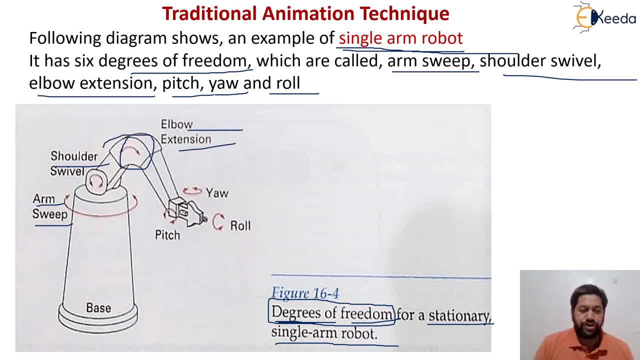 Okay, this is the elbow of the object, So this elbow extension should be rotated in 360 degree Getting in. not only elbow should be rotated, You can find. this is the pitch should be rotated. This yaw should be rotated. this top We are having at the starting point. 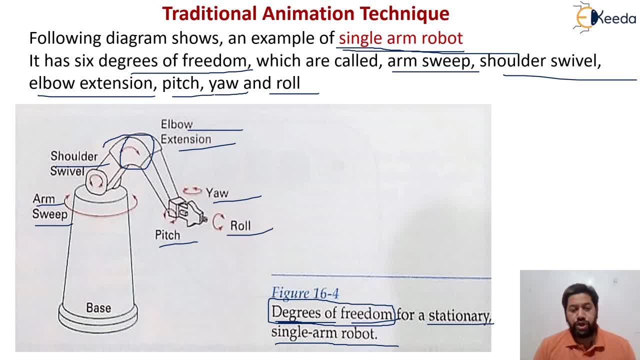 We are having this should be rotated. Okay, so I want the rotation of the all this object should be rotated appropriately, And that is what one of the part of the animation. Okay, So that should be done with the help of the animation and I hope this example. it will clear your concept. 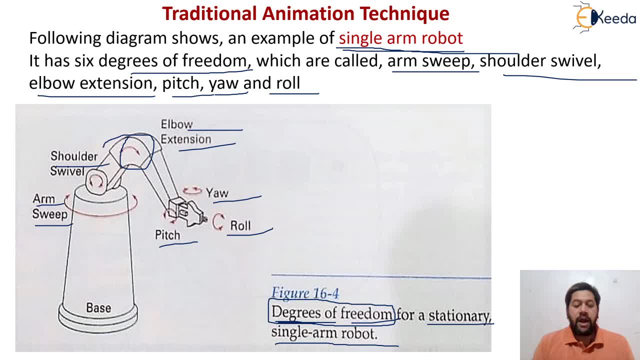 of the traditional animation technique that we are having and what exactly see. our topic of discussion today is introduction to animation. We should understand what is animation, which are the application of the animation, then we should learn which are the animation technique. Okay, I think we have learned. there are the four steps. 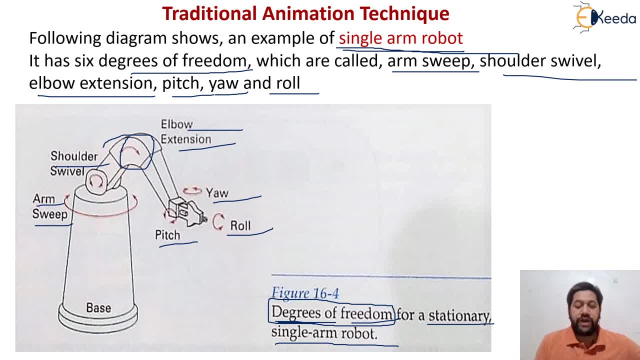 that we have to follow, which is a part of traditional animation technique, which are involved, Okay, And I think we have seen, with help of the diagram also, and all the detail explanation of the techniques which comes under the traditional animation techniques. Okay, I think, with this background, 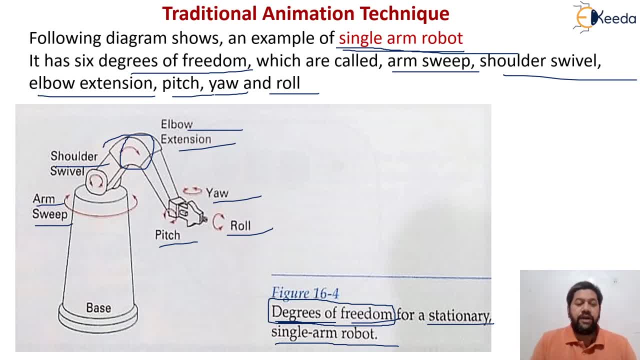 and with all the discussion that we are having. Okay, I think we should end our session here. I hope all of you have understood and enjoyed the session on the introduction to animation and traditional animation techniques. Okay, so I'm going to end my session here. 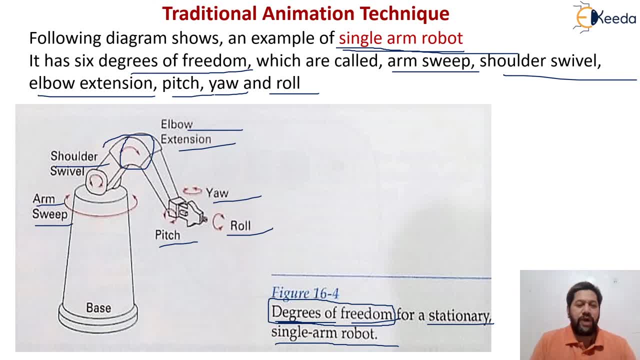 Okay, So thank you for patience listening, Thank you. Thank you, student.